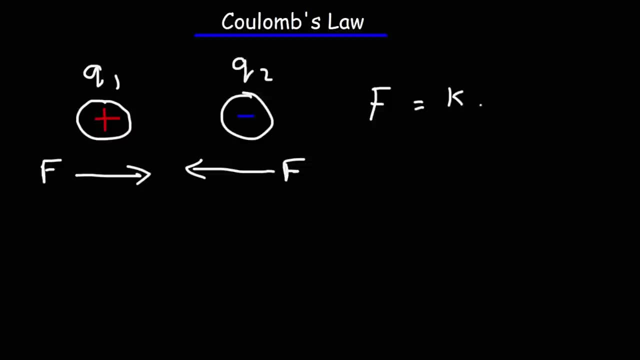 The electric force is equal to the proportionality constant K times the magnitude of Q1 times Q2, divided by R squared Now, R is the distance that the force is going to be applied to. It's the distance between the center of these two charges. 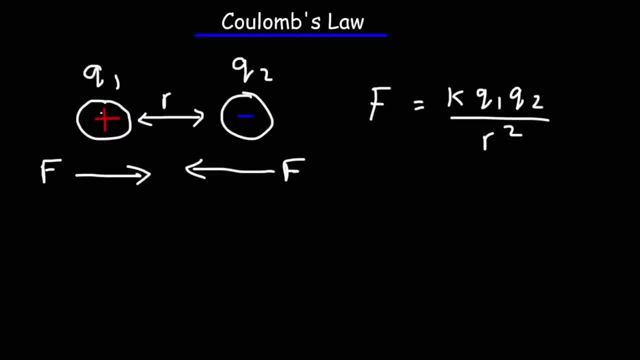 Now these charges are known as point charges, where the size of the charge is irrelevant. The proportionality constant K is equal to 9 times 10, to the 9 Newtons over square meters times square Coulombs. So make sure you know this value because we're going to use it when 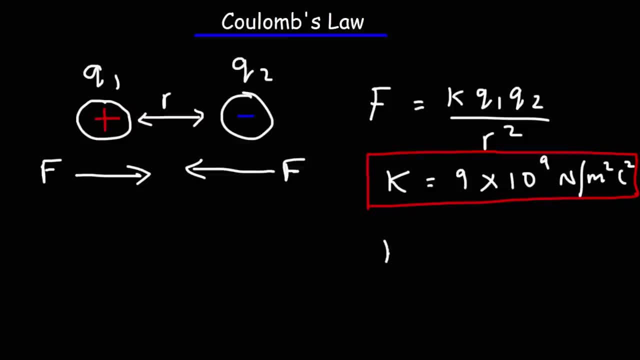 we're solving problems Now. this proportionality constant is always equal to. I mean, it's also equal to 1 over 4 pi times epsilon naught, And epsilon in this problem or in this situation, is equal to 8.85. 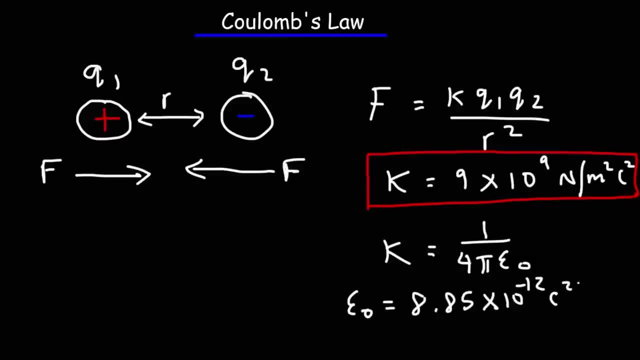 times 10 to the negative, 12 Coulombs squared over Newtons times square meters. So this is the permittivity of free space. Now, when solving problems associated with Coulombs law, K is the value that you're going to use most often. 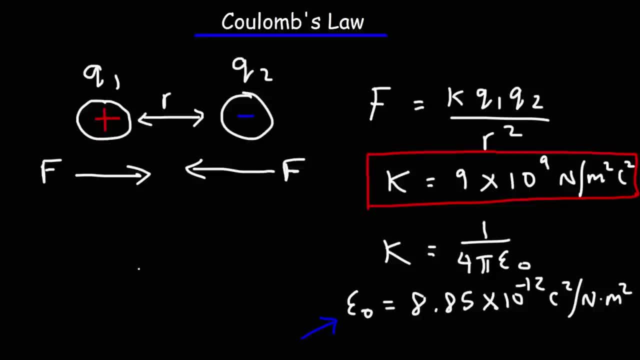 Now we said that opposite charges attract. Let's draw a picture with two light charges. So if we were to put a positive charge next to another positive charge, these two charges will repel, so they will fill a force that will push them apart. but these two forces are. 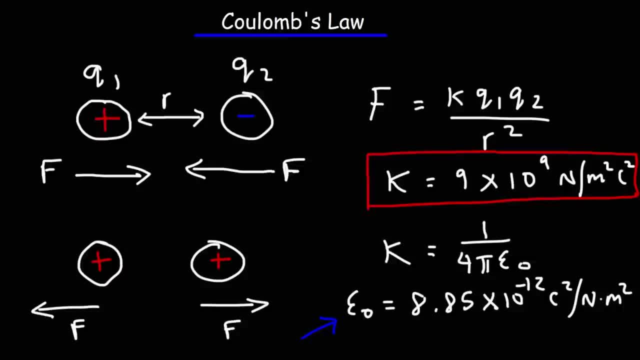 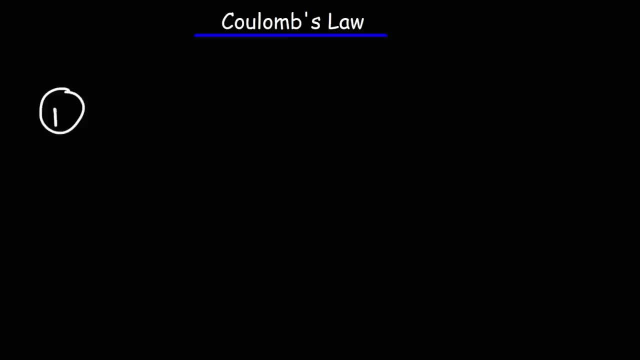 equal in magnitude but opposite in direction. so now to review: remember: protons carry a positive charge and electrons they carry a negative charge. now, whenever you have an object that has a net positive charge, you need to be aware that what it means that is that there's more protons than electrons in. 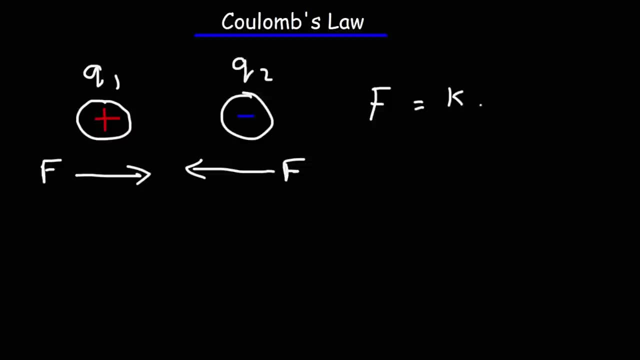 The electric force is equal to the proportionality constant K times the magnitude of Q1 times Q2, divided by R squared Now, R is the distance that the force is going to be applied to. It's the distance between the center of these two charges. 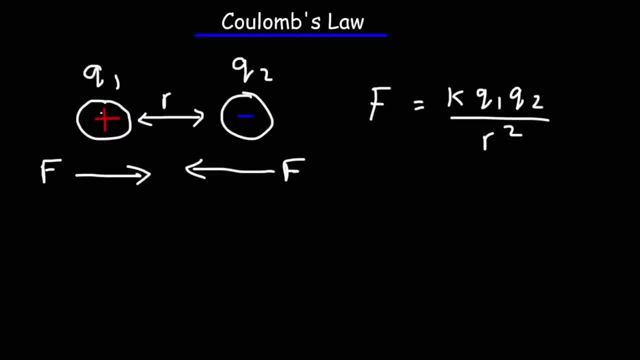 Now these charges are known as point charges, where the size of the charge is irrelevant. The proportionality constant K is equal to 9 times 10, to the 9 Newtons over square meters times square Coulombs. So make sure you know this value because we're going to use it when 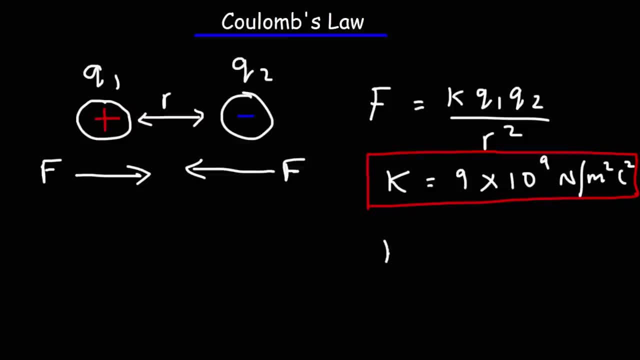 we're solving problems Now. this proportionality constant is always equal to. I mean, it's also equal to 1 over 4 pi times epsilon naught, And epsilon in this problem or in this situation, is equal to 8.85. 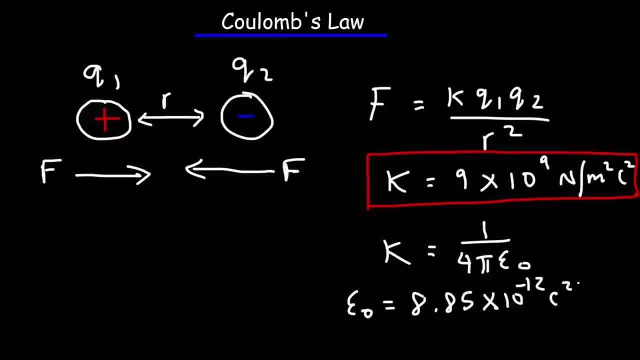 times 10 to the negative, 12 Coulombs squared over Newtons times square meters. So this is the permittivity of free space. Now, when solving problems associated with Coulombs' Law, K is the value that you're going to use most often. 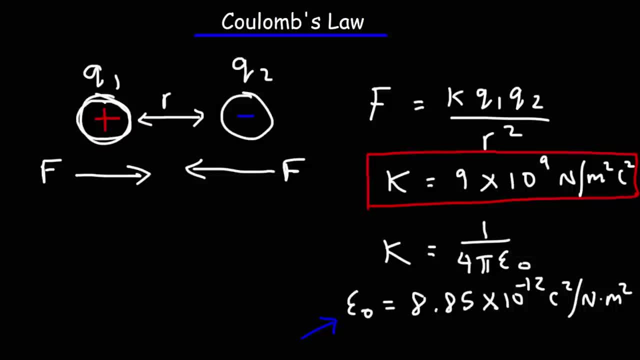 Now we said that opposite charges attract. Let's draw a picture with two light charges. So if we were to put a positive charge next to another positive charge, these two charges will repel, So they will fill a force that will push them apart. 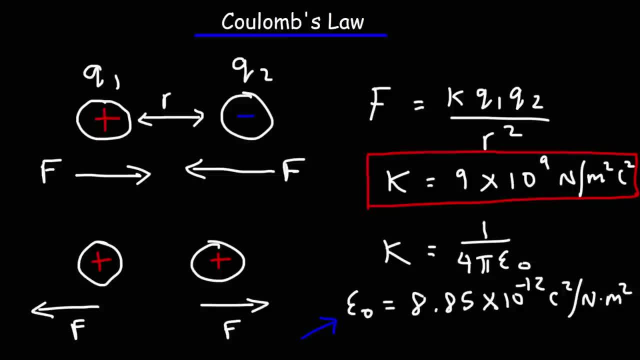 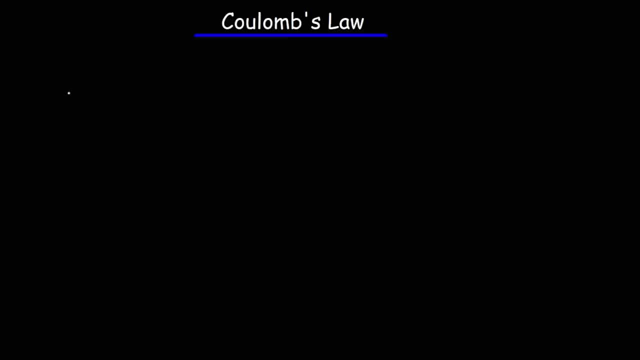 But these two forces are equal in magnitude but opposite in direction. So now to review, remember: protons carry a positive charge and electrons they carry a negative charge. Now, whenever you have an object that has a net positive charge, you need to be aware that what it means is that there's more protons than electrons in that object. 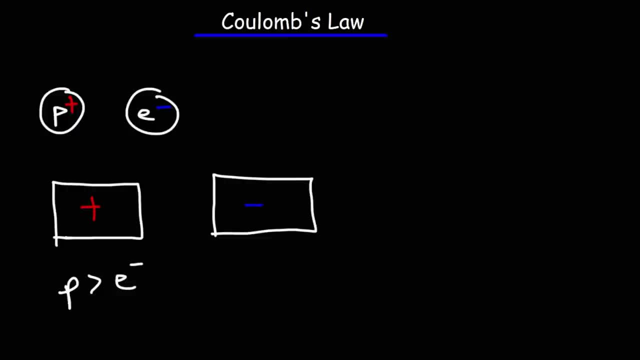 If you have an object that is negatively charged, that means that it has more electrons than protons. So whenever the number of protons and electrons are equal, the object will be negative. The object will be neutral in charge. But if you have more protons than electrons, the object will carry a positive charge. 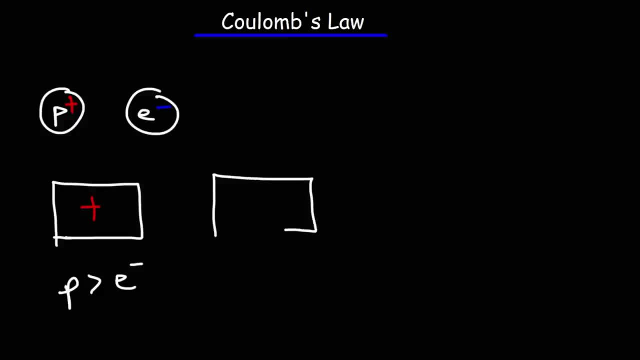 that object. if you have an object that is negatively charged, that means that it has more electrons and protons. so whenever the number of protons and electrons are equal, the object will be neutral in charge. but if you have more protons than electrons, the object will carry a positive charge if there 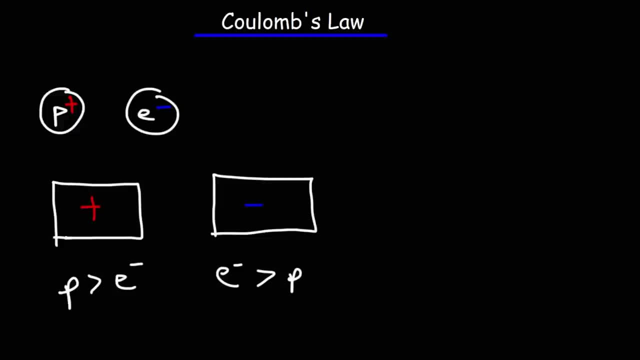 are more electrons than protons, then it's going to have a negative charge. now let's go back to Kaloum's law. This equation describes the relationship between the electrical force, the magnitude of the charges and the distance between it. two charges. If we were to increase the magnitude of 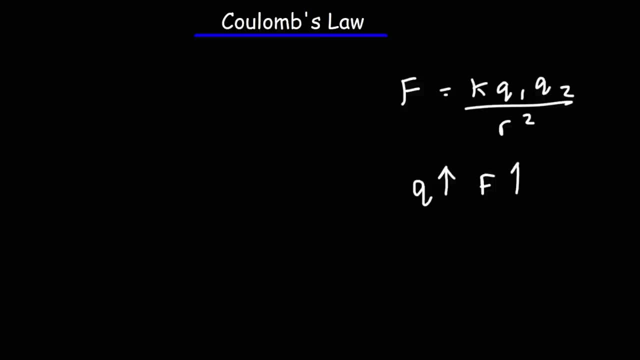 the human body force to one tangent one of the charges, the electric force will increase. So let's say this is Q1 and this is, let's put, a positive charge, and let's say Q2 also has a positive charge, And let's say the force acting on each of them is 100 Newtons. Now, what do? 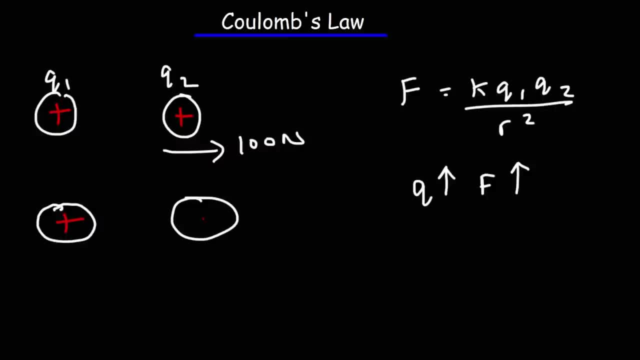 you think is going to happen if we increase the magnitude of one of those charges. Let's say we double the value of Q2. So it's 2 times Q2.. Well, since we increase the magnitude of the charge, the electric force is going to increase. 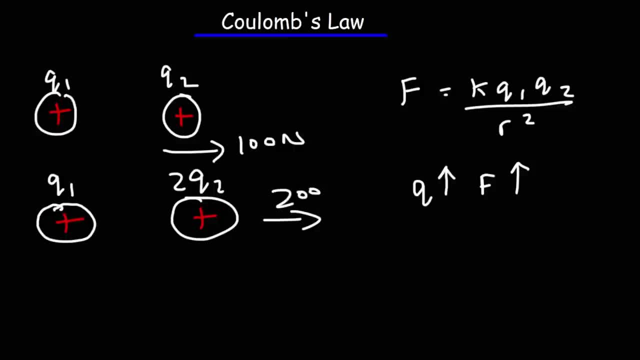 in value, It's going to double. It's going to become 200 Newtons. So if you double the magnitude of one of the charges, the force will double. Now let's say this is R. What happens if we place Q2 further away from Q1?? So let's say, if we double the distance, 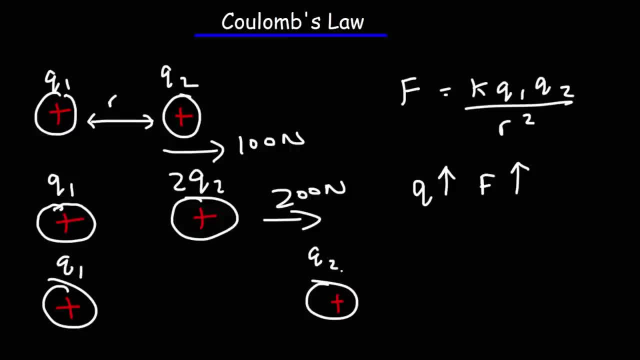 between Q1 and Q2.. So this is going to be 2R instead of 1R. What's going to happen to the force? Notice that R is on the bottom of the fraction. If you were to increase the distance between the two charges, the magnitude of the force will. 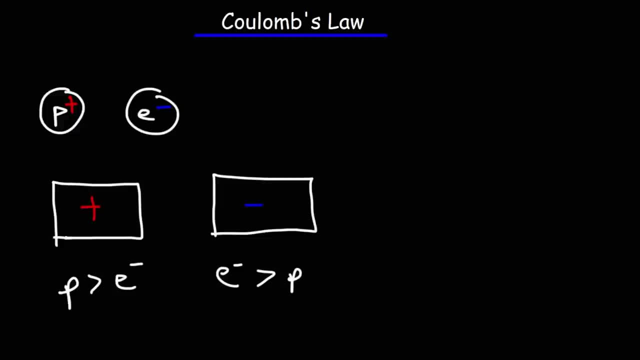 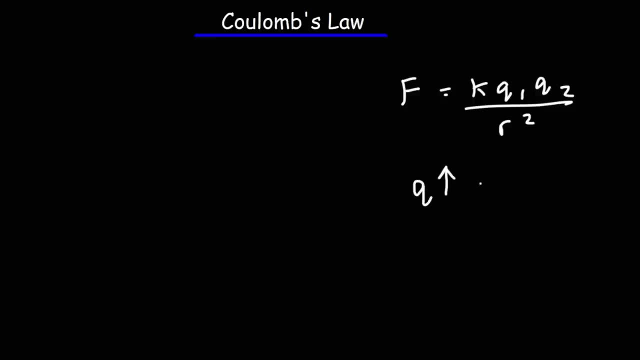 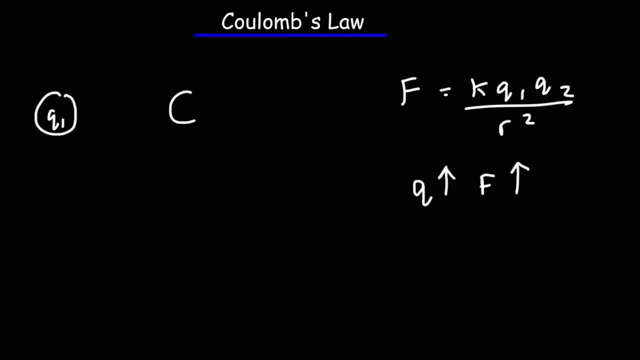 So let's say this is Q1, and this is, let's put, a positive charge. and let's say Q2 also has a positive charge, And let's say the force acting on each of them is 100 Newtons. Now what do you think is going to happen if we increase the magnitude of one of those? 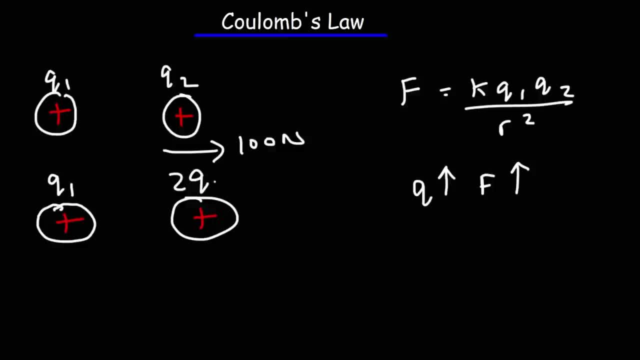 charges. Let's say we double the value of Q2, so it's 2 times Q2.. Well, since we increased the magnitude of the charge, the electric force is going to increase in value. It's going to double. it's going to become 200 Newtons. 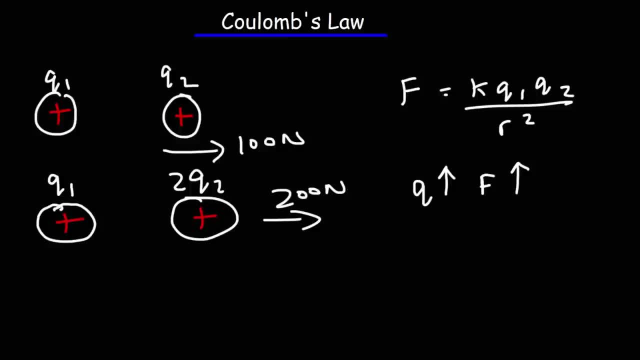 So if you double the magnitude of one of the charges, the electric force is going to increase in value. If you increase the magnitude of one of the charges, the force will double. Now let's say this is R. What happens if we place Q2 further away from Q1?? 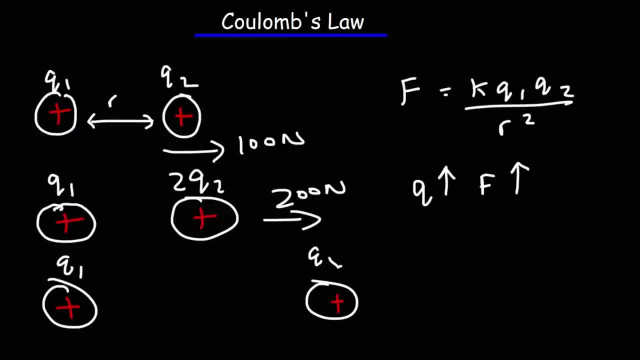 So let's say, if we double the distance between Q1 and Q2, so this is going to be 2R instead of 1R. What's going to happen to the force? Notice that R is on the bottom of the fraction. 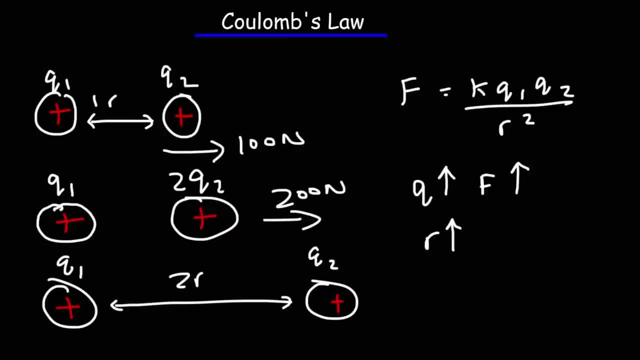 If you were to increase the magnitude of the charge, the electric force is going to increase. If you were to increase the distance between the two charges, the magnitude of the force will decrease. The force is inversely related to the square of the distance. 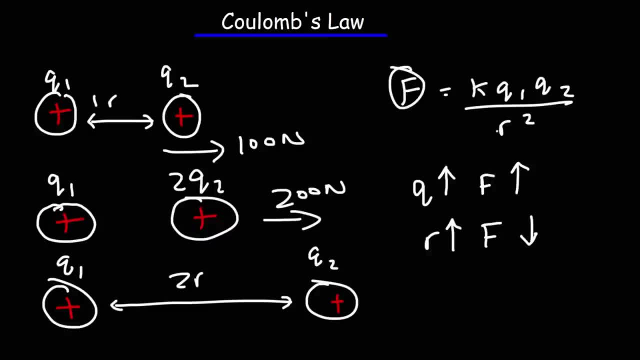 decrease. The force is inversely related to the square of the distance. So the force is not going to cut in half, It's going to be 1 fourth of its original value. Because if you were to plug in 2 into that equation and 1 for everything, 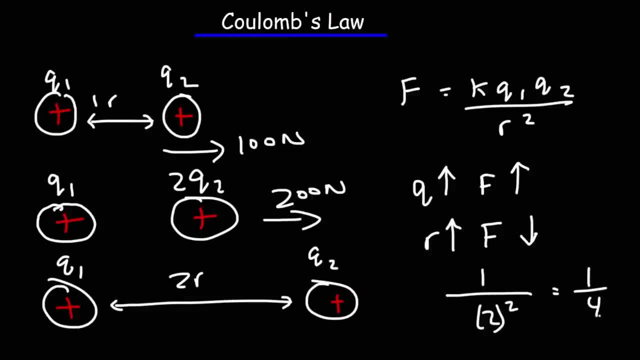 else it would be 1 over 2 squared, which is 1 over 4.. So it's going to be 1 fourth of its original value, which means it's going to be 25 Newtons. So if you were to double the magnitude of one of the charges, the force will double. If 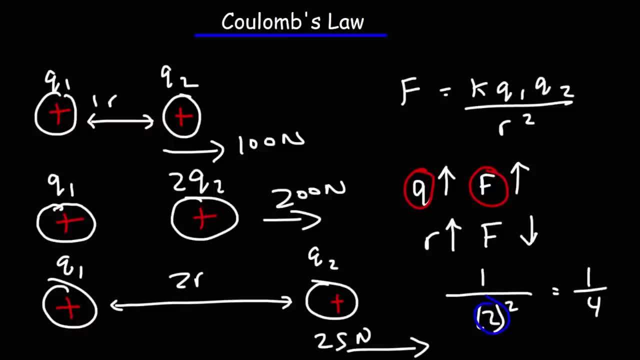 you were to double the distance between the two charges, the force will be reduced by a factor of 4.. So the electric force is strongest when the charges are placed closer together or if you increase the magnitude of the charges. Now let's talk about the units associated with Coulomb's Law. 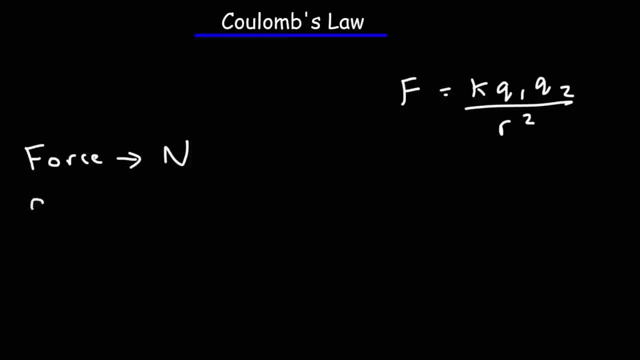 The unit of force is the Newton. Now for Q1 or Q2, which represents the electric charge. the unit for that is Coulombs. One Coulomb is a large amount of charge, So typically you'll see the charge represented in micro-Coulombs: One micro-Coulomb. 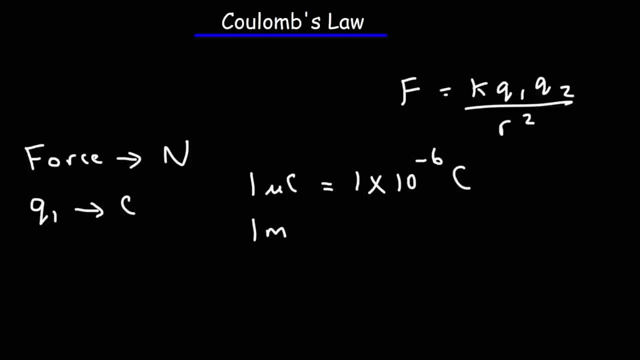 is 1 times 10 to the minus 6 Coulombs, One milli-Coulomb is 1 times 10 to the negative 3 Coulombs, And one nano-Coulomb is 1 times 10 to the minus 6 Coulombs. 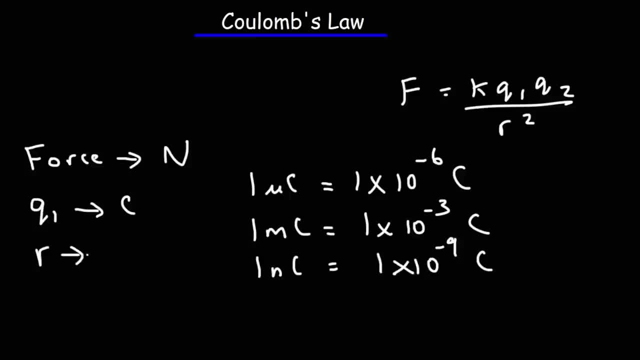 Now R. the distance between the charges needs to be in meters. Sometimes you'll see values in centimeters or millimeter. So remember one centimeter is 1 times 10 to the minus 2 meters, And one millimeter is 1 times 10 to the minus 3 meters. You 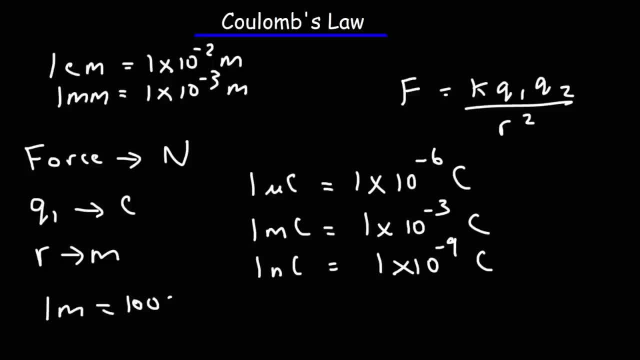 could also see it this way: One meter is equivalent to 100 centimeters And one milli- I mean one meter- is equivalent to 1000 millimeters. So those are some other things that you want to know when dealing with problems associated with Coulomb's Law. 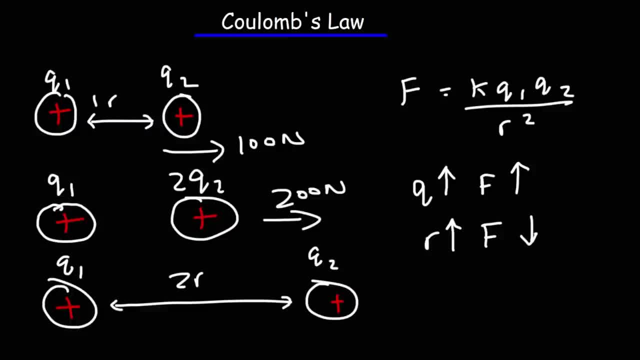 So the force is not going to cut in half, it's going to be 1 fourth of its original value, Because if you were to plug in 2 into that equation and 1 for everything else, it'd be 1 over 2 squared, which is 1 over 4.. 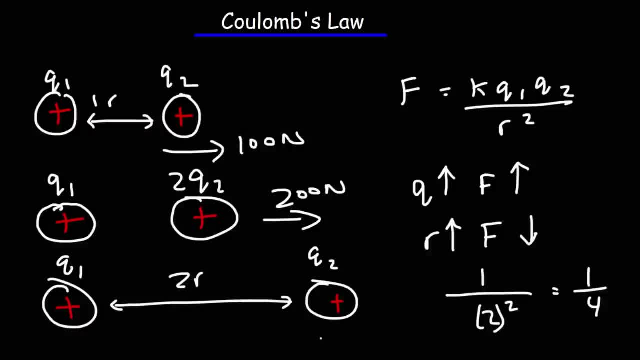 So it's going to be 1 fourth of its original value, which means it's going to be 25 newtons. So if you were to double the magnitude of one of the charges, the force will double. If you were to double the distance between the two charges, the force will be reduced. 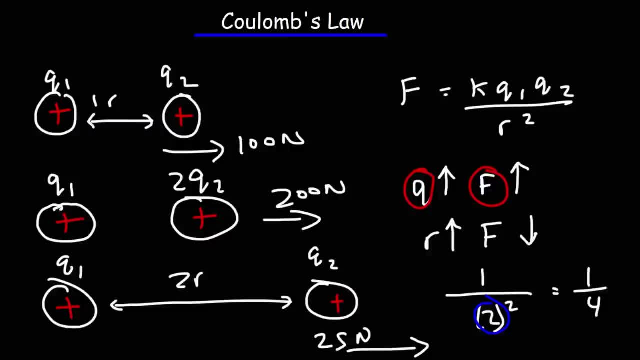 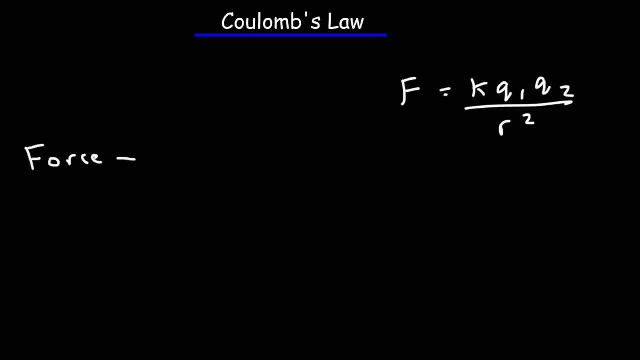 by a factor of 4.. So the electric force is strongest when the charges are placed closer together or if you increase the magnitude of the charge. Now let's talk about the units associated with Coulomb's Law. The unit of force is the newton. 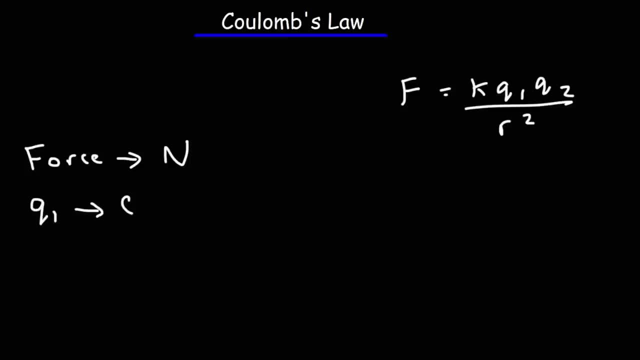 Now for Q1 or Q2, which represents the electric charge. the unit for that is Coulombs. One Coulomb is a large amount of charge, So typically you'll see the charge represented in micro-Coulombs. One micro-Coulomb is 1 times 10 to the minus 6 Coulombs. 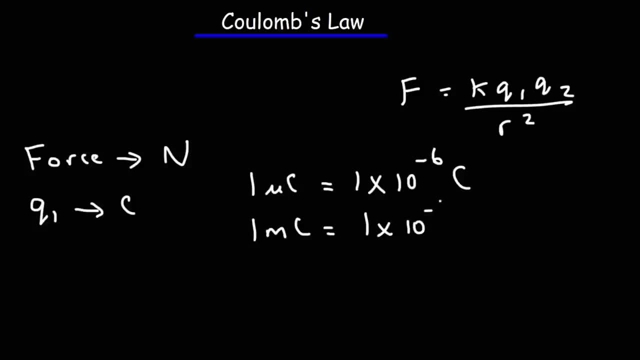 One mili-Coulomb is 1 times 10 to the negative 3 Coulombs, And one nano-Coulomb is 1 times 10 to the negative 9 Coulombs. Now R? the distance between the charges needs to be in Meters. 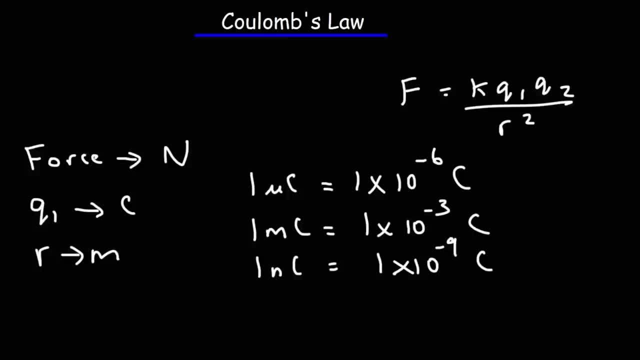 Sometimes you'll see values in centimeters or millimeters, So remember one centimeter is 1 times 10 to the minus 2 Meters. So R is 1 times 10 to the minus 2 Meters And 1 mm is 1 times 10 cubed. 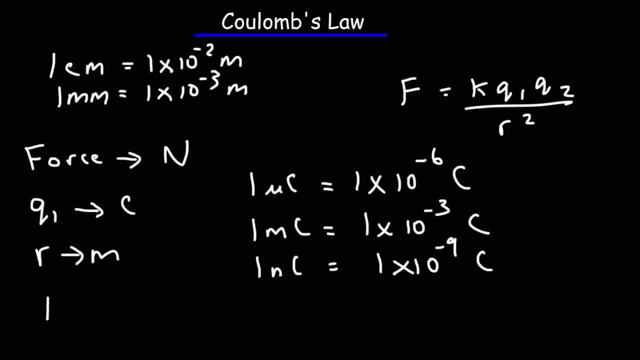 Remember, your placebo range can vary the reaction time of your charge. Yes, 10 to the minus 3 meters. you could also see it this way: one meter is equivalent to 100 centimeters and one million- i mean one meter- is equivalent to a thousand millimeters. so those are some other. 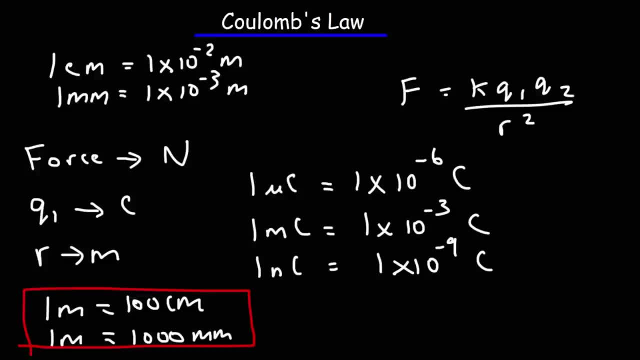 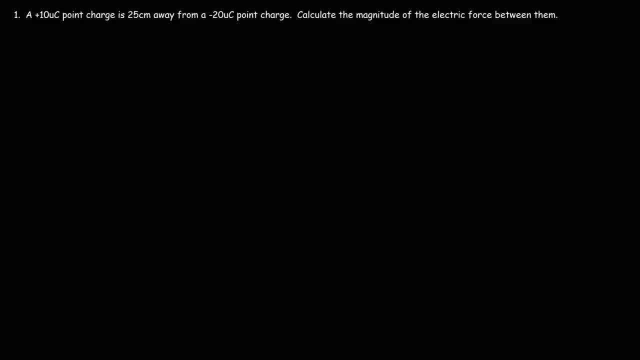 things that you want to know when dealing with problems associated with klum's law. now let's work on some practice problems. let's start with this one. a 10 microcoulomb point charge is 25 centimeters away from a negative 20 microcoulomb point charge. 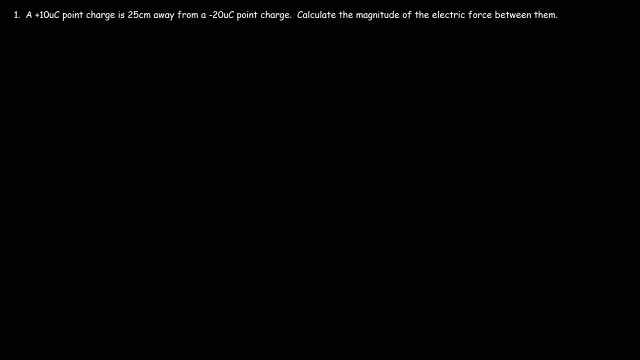 Now let's work on some practice problems. Let's start with this one: A 10 micro-Coulomb point charge is 25 centimeters away from a negative 20 micro-Coulomb point charge. Calculate the magnitude of the electric force between them. So let's begin by 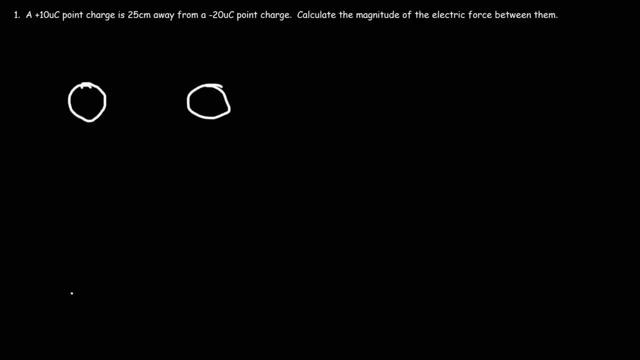 drawing a picture. So we have two charges. One is positive, The other is negative. We'll call this Q1 and Q2.. So Q1 has a magnitude of positive: 10 micro-Coulombs, Q2 has a magnitude of negative: 20 micro-Coulombs, And the distance between the two charges is 25 centimeters. 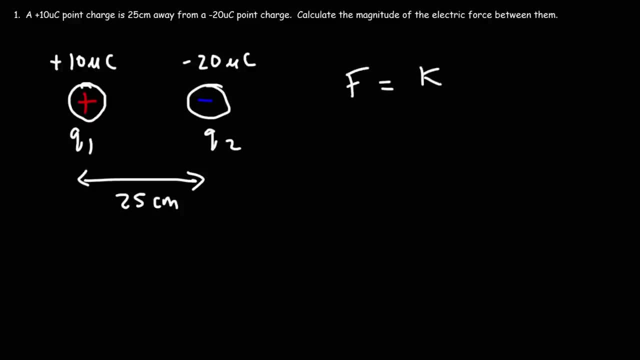 So now let's calculate this, Calculate the force acting on the two charges. Now keep in mind: since we're dealing with opposite charges, these two will feel a force of attraction, So these two forces will be equal in magnitude. The force that is acting on charge 1 due to charge 2, you can call 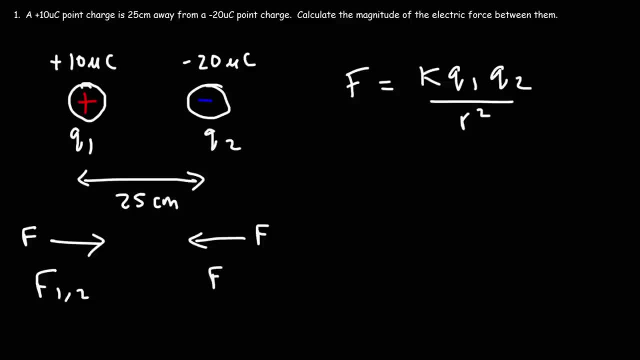 it F1 comma 2.. The force that is acting on charge 2 due to charge 1, you can call it F2 comma 1.. But for this problem they're exactly the same. Now the proportionality constant K is 9 times 10 to the 9.. Q1 is 10 micro-Coulombs. 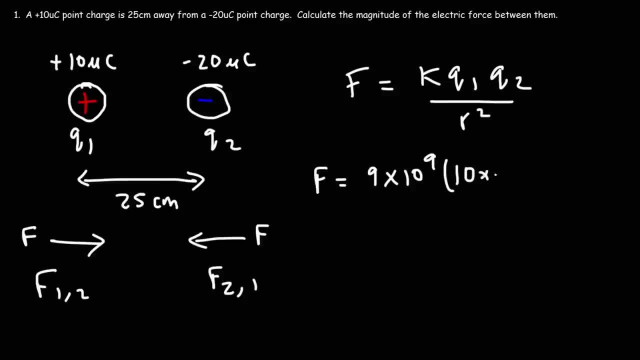 So to plug this in, replace micro-Coulombs with 10 to the negative: 6 Coulombs. Q2 is negative: 20 micro-Coulombs. Now for this formula. you don't need to worry about the negative sign, Because we already know the direction of the formula. 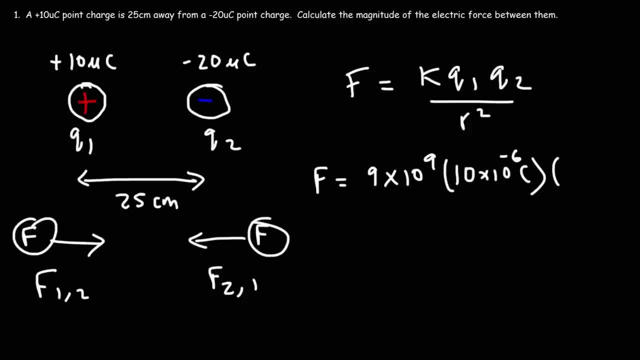 Now for this formula. you don't need to worry about the negative sign, Because we already know the direction of the formula, Because we already know the direction of the formula force. Also, we only want the magnitude of the electric force. Electric force is a vector. It. 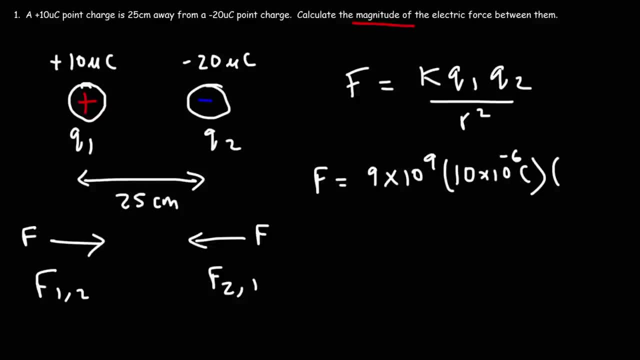 has both magnitude and direction. but since we only want the magnitude, we don't need to be concerned with the direction and we don't need to worry about the negative sign. So we're going to plug in positive 20 times 10 to the minus 6 coulombs for Q2.. Now R, the distance between the 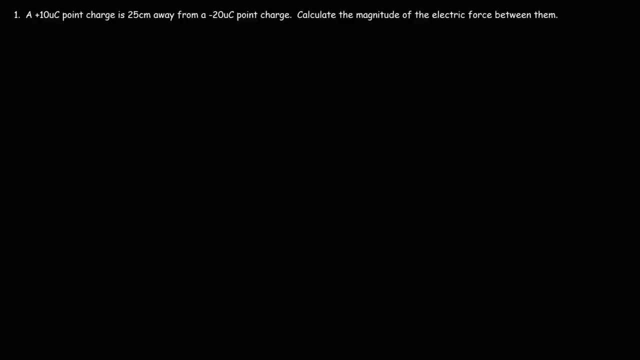 calculate the magnitude of the electric force between them. so let's begin by drawing a picture. so we have two charges, one is positive, the other is negative. we'll call this q1 and q2. so q1 has a magnitude of positive, 10 microcoulombs, q2 has a magnitude of negative, 20 microcoulombs, and the distance between 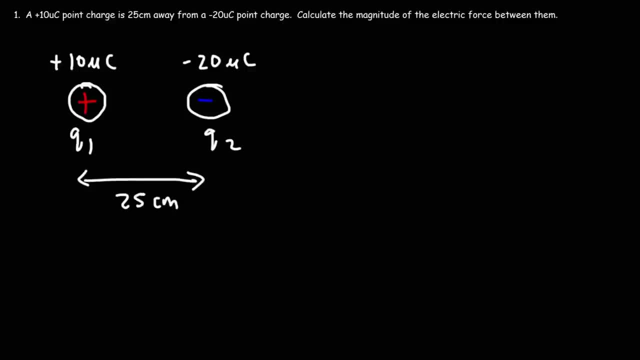 the two charges is 25 centimeters. so now let's calculate the force acting on the two charges. now keep in mind, since we're dealing with opposite charges, these two will fill a force of attraction, so these two forces will be equal in magnitude. the force that is acting on charge one due to charge two- you can call it f one comma two. 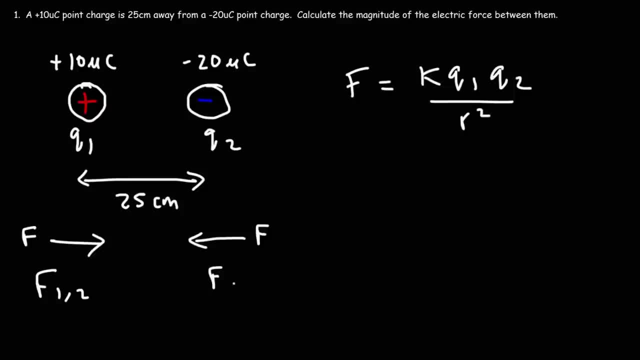 the force that is acting on charge two due to charge one. you can call it f two comma one, but for this problem they're exactly the same. now the proportionality constant k is nine times ten to the nine. q1 is 10 microcoulombs. 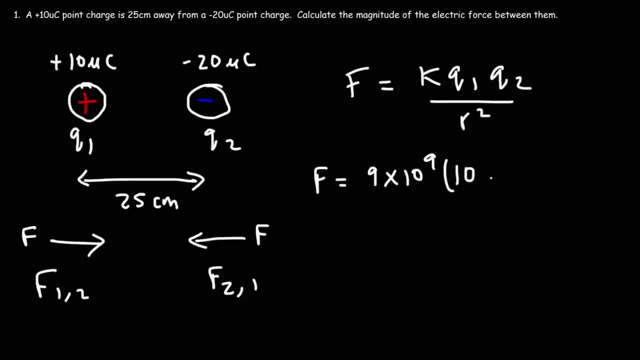 it's going to be 10 to the minus three, 20 microcoulombs. so to plug this in, replace microclomes with 10 to the negative 6 columns. q2 is negative 20 microclomes. now for this formula, you don't need to worry about the negative sign, because we already know the direction of the force. 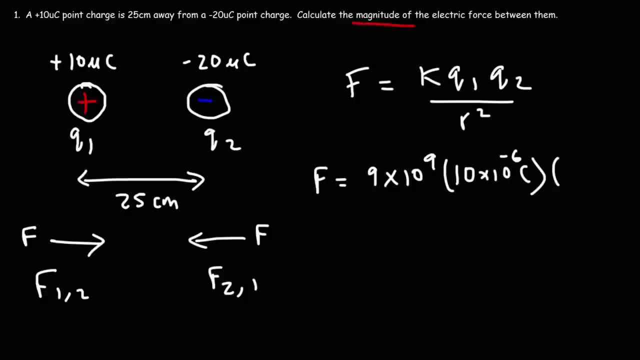 also, we only want the magnitude of the electric force. electric force is a vector. it has both magnitude and direction. but since we only want the magnitude, need to be concerned with the direction and we don't need to worry about the negative sign. So we're going to plug in positive 20 times 10 to the minus 6 coulombs for Q2.. 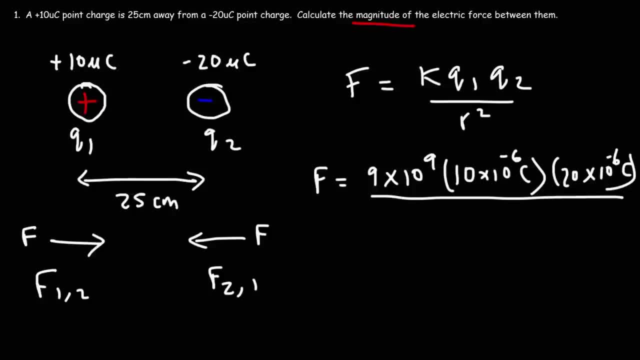 Now R. the distance between the two charges is in centimeters. We need to convert that to meters. Well, actually you can simply plug it in like this: 25 centimeters. you can write it as 25 times 10 to the minus 2 meters. You can replace centi with 10 to negative 2.. 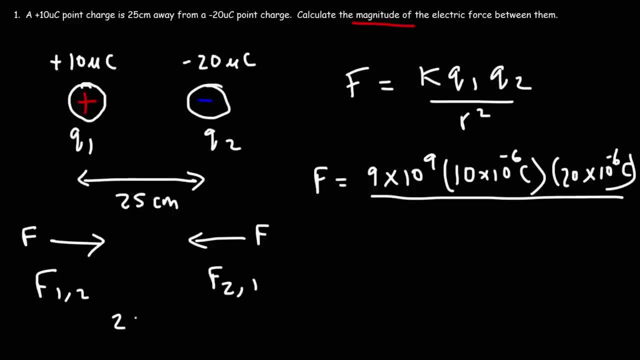 two charges is in centimeters. We need to convert that to meters. Well, actually you can simply plug it in like this: 25 centimeters. you can write it as 25 times 10 to the minus 2 meters You can. 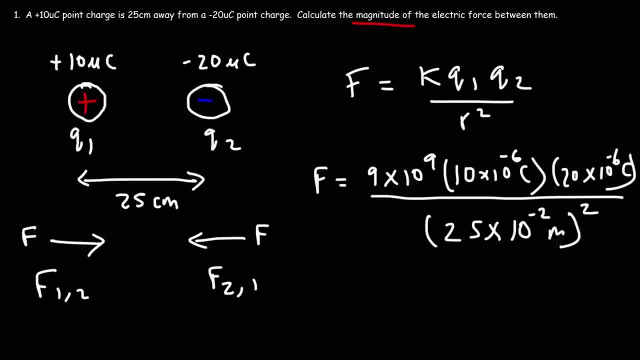 replace centi with 10 to negative 2.. But if you wanted to convert it, here's what you could do: You can multiply 25 centimeters by 1 meter over 0.5 centimeters. So you can multiply 25 centimeters by 1 meter over 0.5 centimeters. 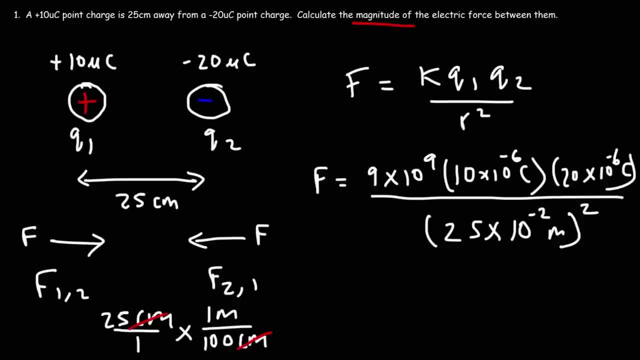 And this will give you 0.25 meters when you divide 25 by 100.. Or you can move the decimal point 2 units to the left. That will give you 0.25 meters, which is the same as 25 times 10. to the negative. 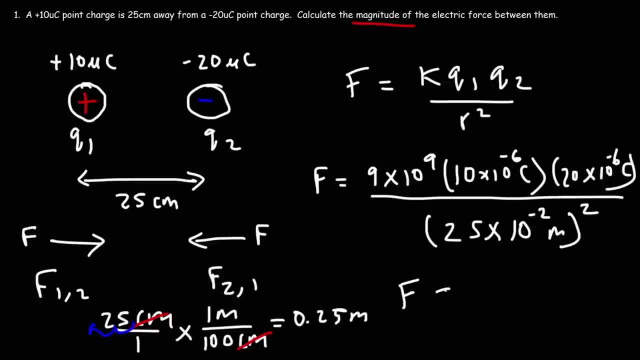 2. So let's go ahead and plug everything in: 9 times 10 to the 9 times 10 times 10 to the minus 6 times the other number divided by and for this part you want to put it in parentheses- You can divide. 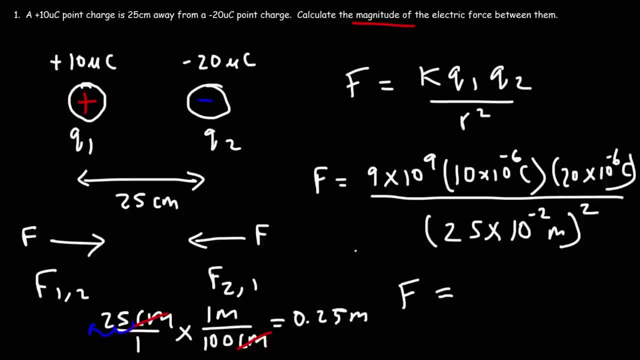 it by 0.25 squared, if you want to, or type in exactly what you see here. So the answer that you should get is 28.8 newtons. So that is the magnitude of the electric force that is acting on both of the two charges. Now let's move on to number two, The electric force between: 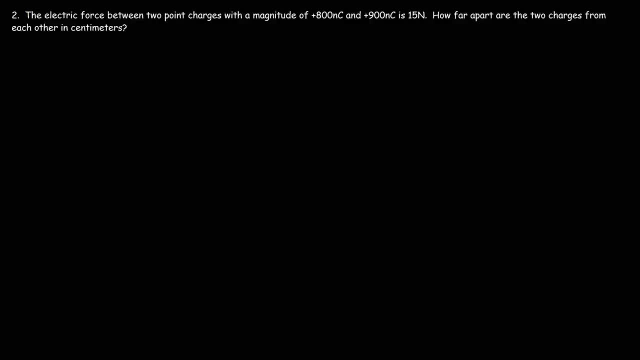 two point charges with a magnitude of 800 nanoclones and 900 nanoclones is 15 newtons. How far apart are the two charges from each other in centimeters? So we can draw another picture if we want to. So here's the first charge and here's the second charge, Both 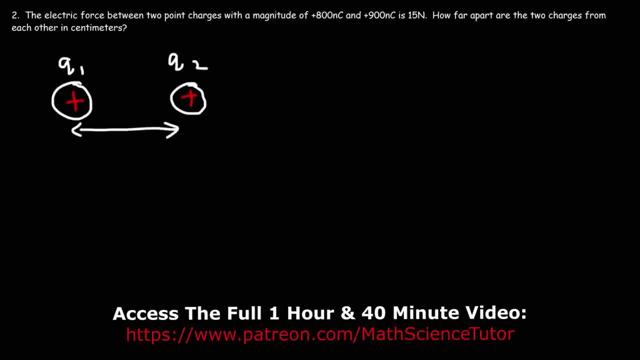 of the two charges are positive, We need to calculate the distance between them, And we know the force acting on each of them. Now, because these two have the same charges, they will repel each other with a force of 15 newtons. But how can we calculate R? Well, let's start with Coulomb's Law. F is 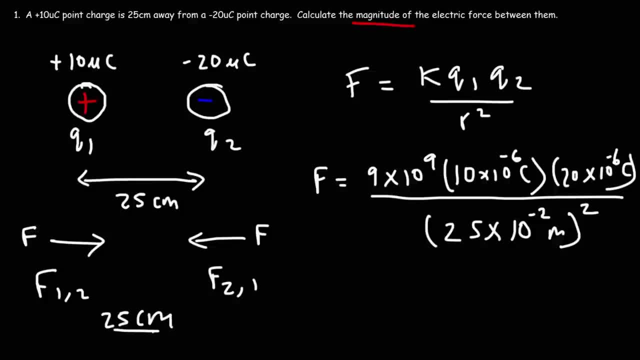 But if you wanted to convert it, here's what you could do: You can multiply 25 centimeters by 1 meter over 100 centimeters, And this will give you 0.25 meters when you divide 25 by 100. Or you can move the decimal. 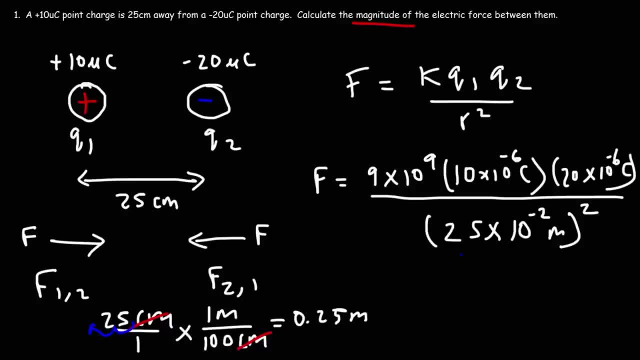 point 2 units to the left, That will give you 0.25 meters, which is the same as 25 times 10 to the negative 2.. So let's go ahead and plug everything in: 9 times 10 to the 9, times 10, times 10 to the minus 6, times the other number. 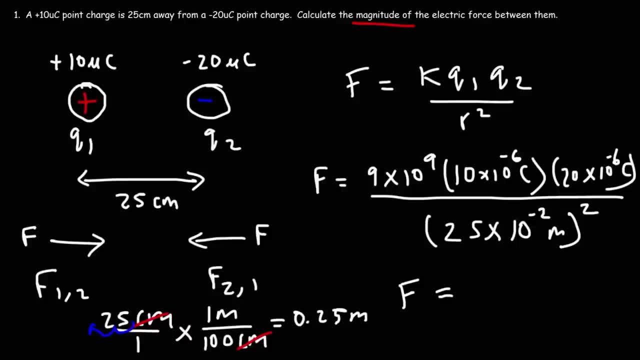 divided by- and for this part, you want to put it in parentheses. You can divide it by 0.25 squared if you want to, or type in exactly what you see here. So the answer that you should get is 28.8 newtons. 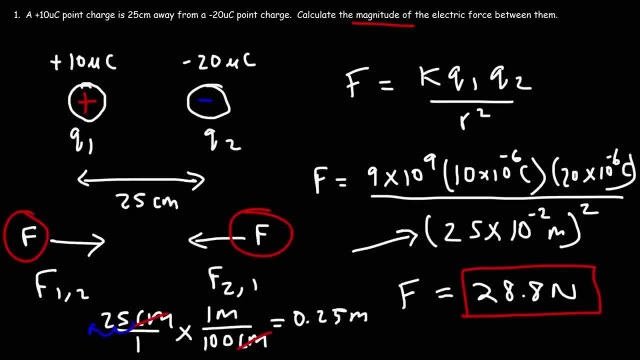 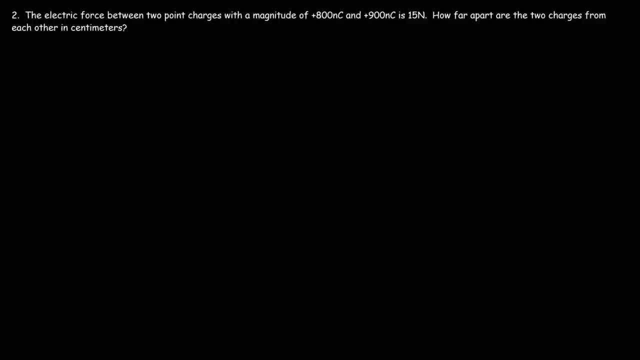 So that is the magnitude of the electric force that is acting on both of the 2 charges. Now let's move on to number 2.. The electric force between 2 point charges with a magnitude of 800 nanokloons and 900 nanokloons is 15 newtons. 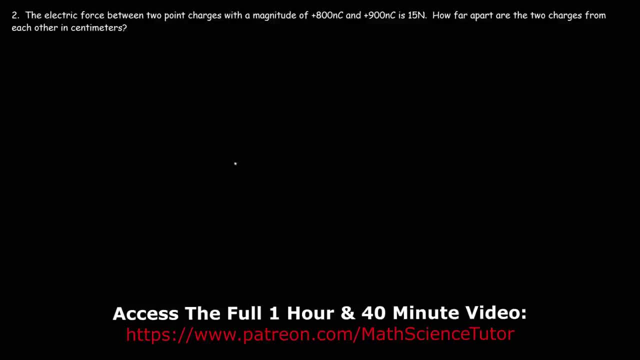 How far apart are the 2 charges from each other in centimeters? So we can draw another picture if we want to. So here's the first charge and here's the second charge. Both of the two charges are positive. We need to calculate the distance between them and we know the force acting on each. 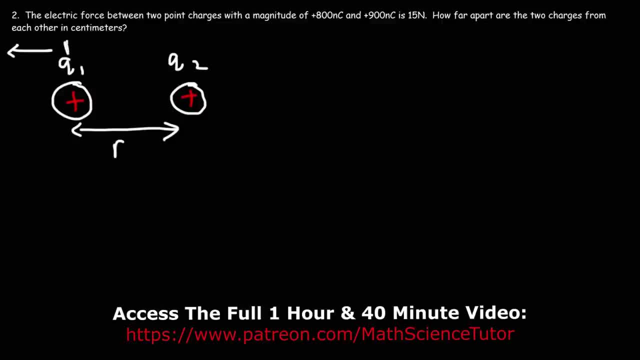 of them Now, because these two have the same charges, they will repel each other with a force of 15 Newtons. But how can we calculate r? Well, let's start with Coulomb's Law. F is equal to kq1 times q2 over r squared. 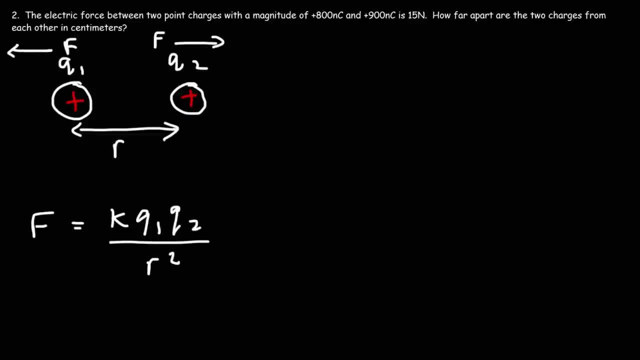 So what we're going to do is we're going to isolate r in this equation. So to do that, let's multiply both sides by r squared first, So these will cancel and we're going to get f times r squared. So this will give us: r squared is equal to kq1q2 over f. 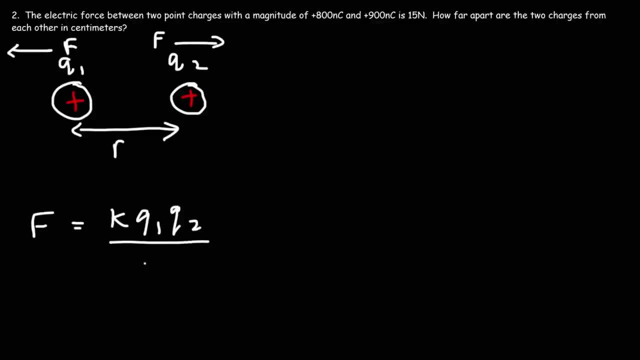 equal to K Q1 over Q2, I mean K Q1 times Q2 over R squared. So what we're going to do is we're going to isolate R in this equation. So to do that, let's multiply both sides by. 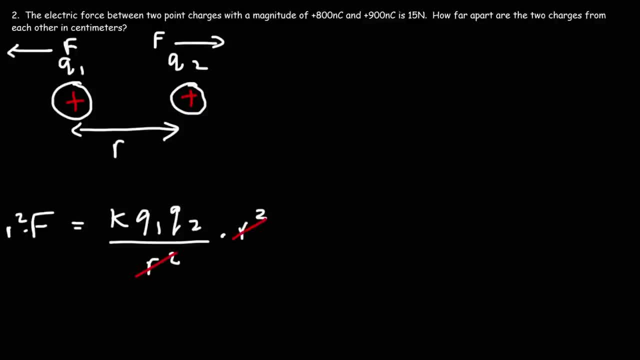 R squared, So these will cancel And we're going to get F times. R squared is equal to K, Q1, Q2.. Now let's divide both sides by F, So this will give us: R squared is equal to K, Q1, Q2 over. 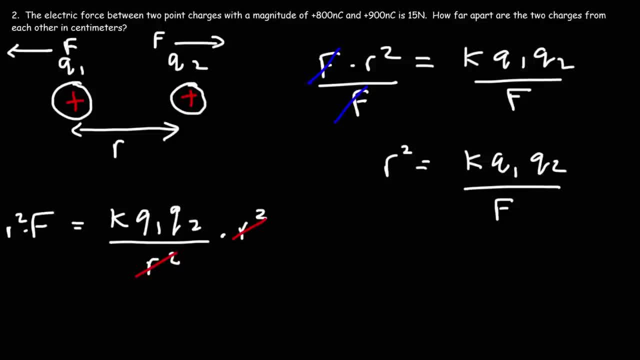 F. Now, to get R by itself, we need to take the square root of both sides. So we're going to do that by doing this. That is equal to Q3 times R. squared is equal to R squared does make P. and then we're going to multiply both sides by Q2 squared. Now acting on both sides. 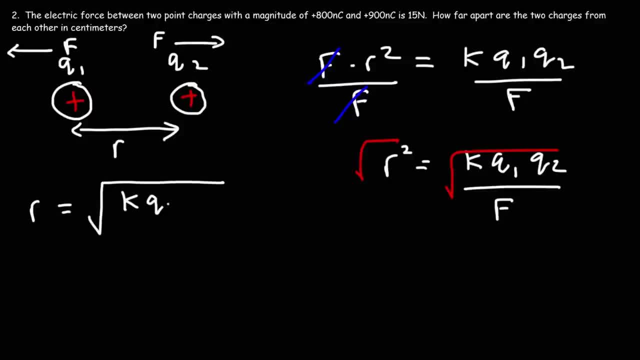 on this, honestly, we're going to get queen and we're going to get very smart alphabets or a square root. So phase two is the entarrement重 offset. So now the test. all of the times is positive. 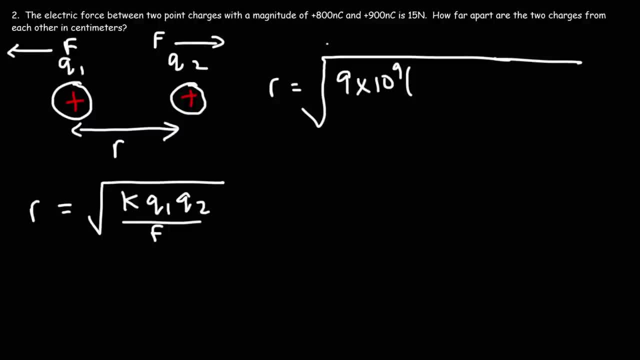 All right, it really doesn't matter which one is Q1, so let's just make this one Q1 and the other one Q2.. Q1 is 800 nanoclombs. keeping in mind nano is 10 to the minus 9.. 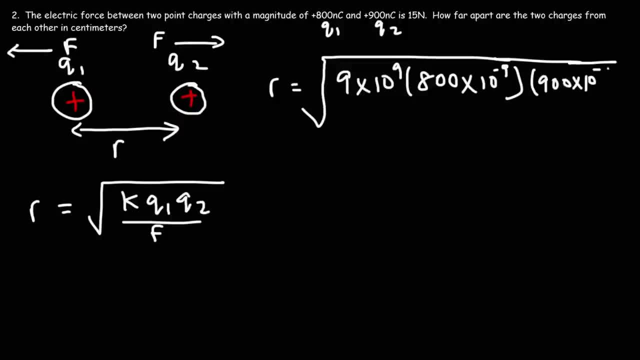 Q2 is 900 nanoclombs, so 900 times 10 to the minus 9.. And then F is 15 newtons. Now, for those of you who want to see the units K, I'm going to plug in the units in this formula. 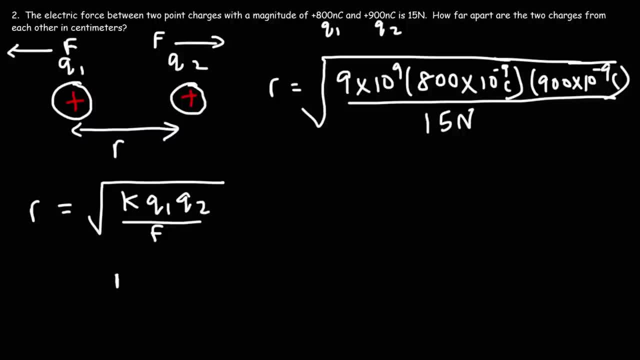 K has the units newtons over square meters. square clombs. Q1 is in clombs, Q2 is in clombs, F is in newtons, So the unit newtons cancel, The unit clombs cancels. So we have square meters. 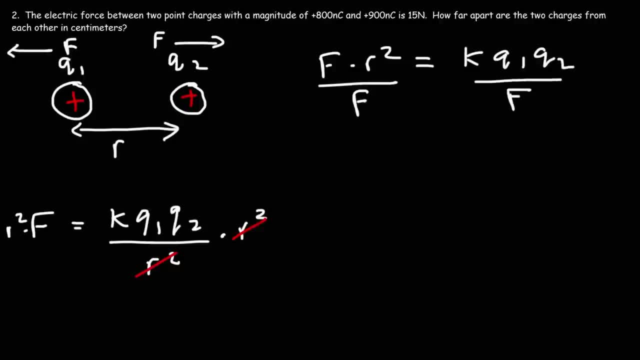 Now let's divide both sides by f, So this will give us r squared is equal to kq1q2 over f. Now to get r by itself, we need to take the square root of both sides. So this is the formula that we can use to calculate the radius, or not really the radius. 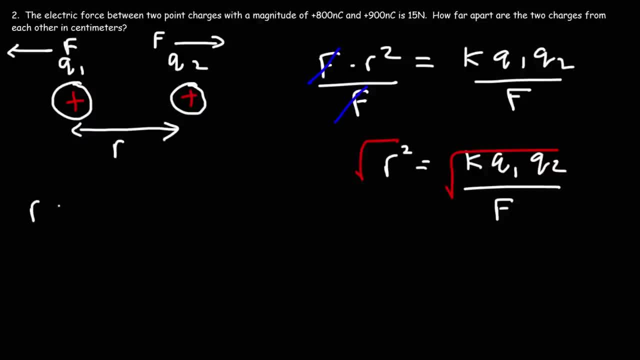 but- I think of the radius when I see r, but the distance between the two charges. So R is going to equal the square root of KQ1 times Q2 divided by F. So K is 9 times 10 to the 9.. 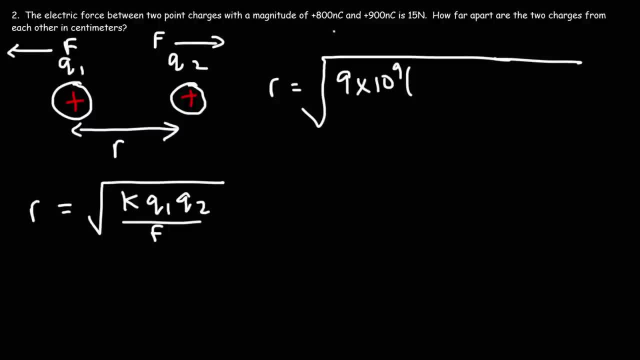 Q1,. it really doesn't matter which one is Q1, so let's just make this one Q1 and the other one Q2.. Q1 is 800 nanoclumes. keeping in mind nano is 10 to the minus 9.. 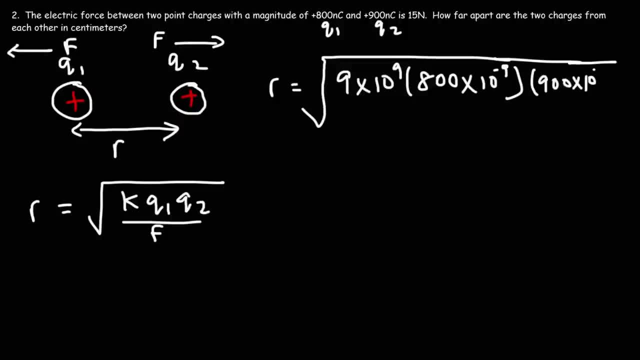 Q2 is 900 nanoclumes, so 900 times 10 to the minus 9.. And then F is 15 newtons. Now, for those of you who want to see the units K, I'm going to plug in the units in this form. 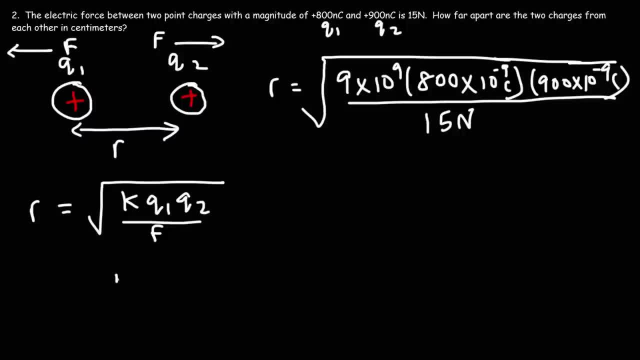 K has the units newtons over square meters. square clumes. Q1 is in clumes, Q2 is in clumes, F is in newtons, So the unit newtons cancel, the unit clumes cancels. so we have square meters. 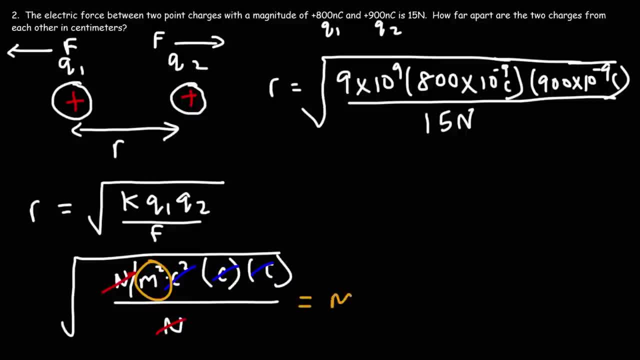 And when you take the square root of square meters, you're going to get the answer in meters. For those of you who want to see how the units work in that formula, Now let's go ahead and plug in these values into a calculator so we can get our final answer. 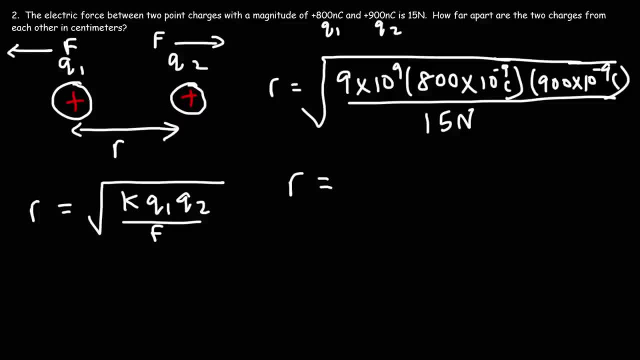 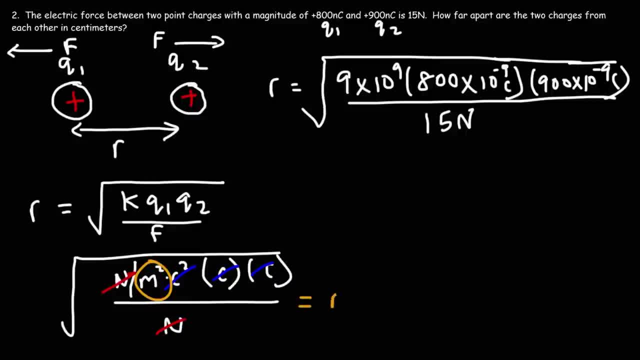 And when you take the square root of square meters, you're going to get the answer in meters. For those of you who want to see how the units work in that formula, Now let's go ahead and plug in these values into a calculator so we can get our final answer. 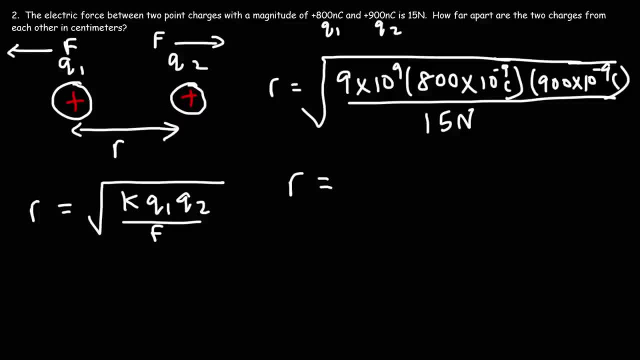 So let's plug in the square root of 9 times 10 to the 9, times 800 times 10 to the 9, times 900 times 10 to the minus 9, divided by 15.. So you should get this answer. 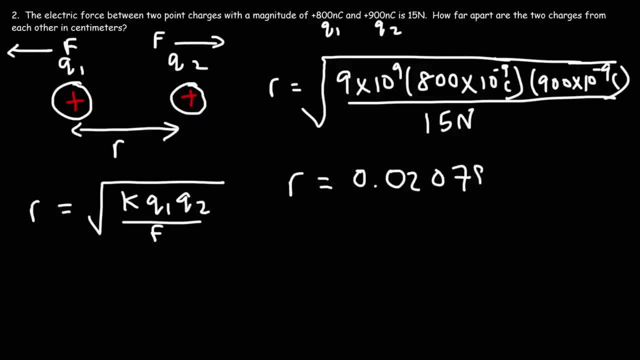 0.02078 meters. Now let's go ahead and convert that to centimeters, Because we want the answer to be in centimeters. Now remember, 1 meter is equivalent to 100.. So you want to set up the conversion in such a way that the unit meters cancel. 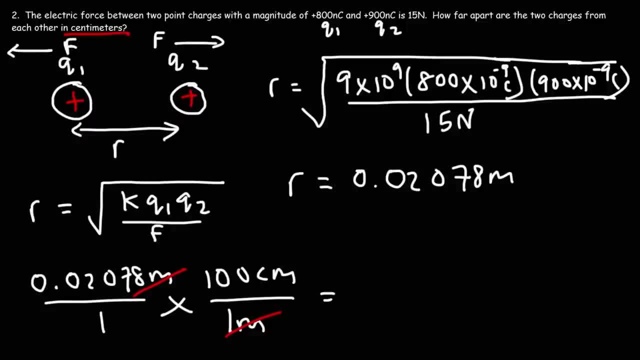 So we're going to multiply 0.02078 by 100.. Or simply move the decimal two units to the right, So we're going to get 2.078 centimeters. So that's the distance between the two point charges Number 3.. A force of 500 newtons exists between 2.078 and 2.078.. So that's the distance between the two point charges. So that's the distance between the two point charges. So that's the distance between the two point charges. 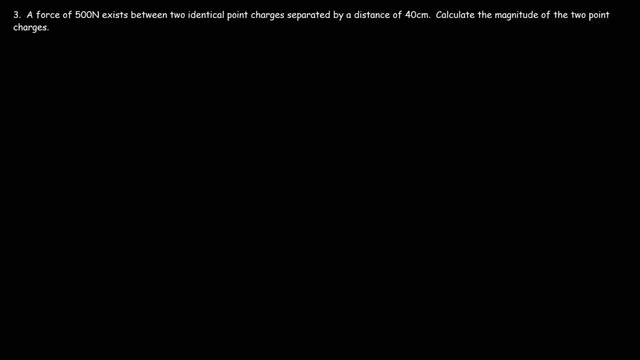 So that's the distance between the two identical point charges, separated by a distance of 40 centimeters. Calculate the magnitude of the two point charges. So let's draw a picture. So here are the two point charges. They're identical. They can both be positive or both be negative. 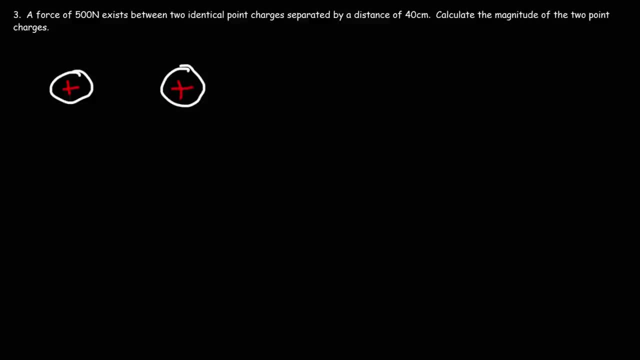 Now, because they're identical, we don't have to describe them as Q1 and Q2.. We can simply refer to them as Q because they're the same. as the problem mentions, they are identical. now we know the distance between the two point charges, and so that is our R value, which is 40. 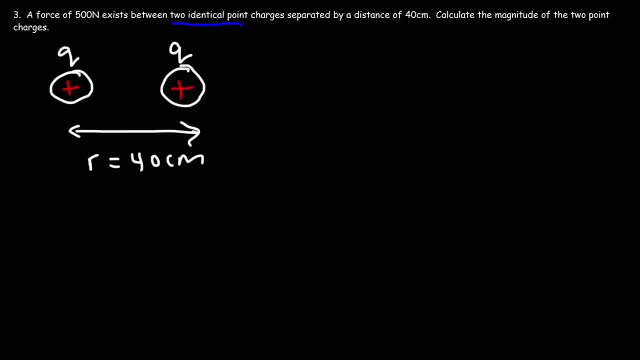 centimeters. now we want to convert that to meters. so to quickly convert centimeters to meters, simply divide by 100 or move the decimal two units to the left. so 40 centimeters is equivalent to 0.40 or 0.4 meters. now we have the. 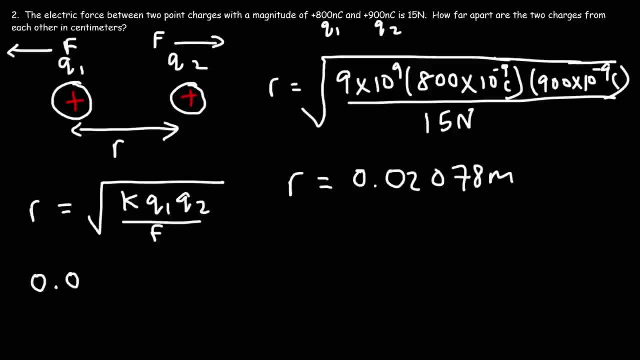 Now let's go ahead and convert that to centimeters, because we want the answer to be in centimeters. Now remember, one meter is equivalent to 100 centimeters, So you want to set up the conversion in such a way that the unit meters cancel. 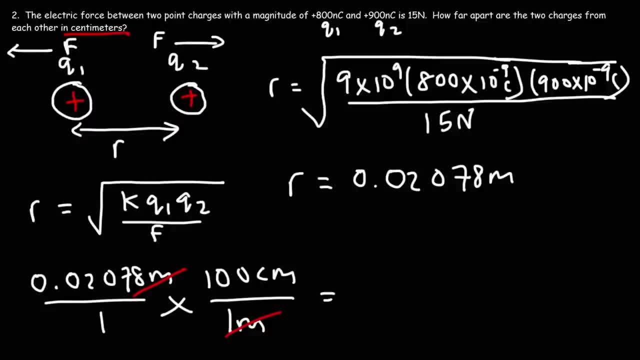 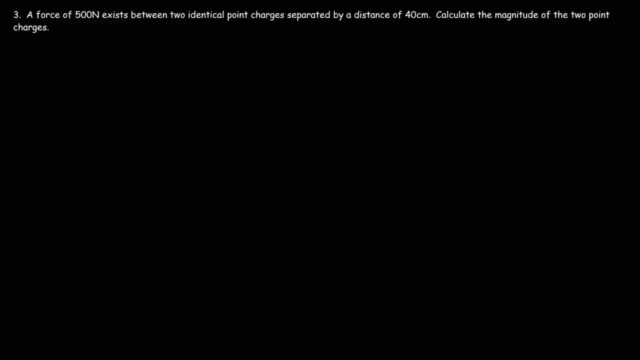 So we're going to multiply 0.02078 by 100. Or simply move the decimal two units to the right, So we're going to get 2.078 centimeters. So that's the distance between the two point charges. Number three: a force of 500 newtons exists between two identical point charges separated by a distance of 40 centimeters. 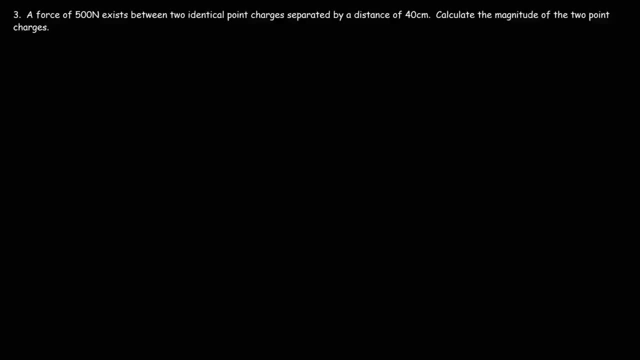 Calculate the magnitude of the two point charges. So let's draw a picture. So here are the two point charges. They're identical. They can both be positive or both be negative. Now, because they're identical, we don't have to describe them as Q1 and Q2.. 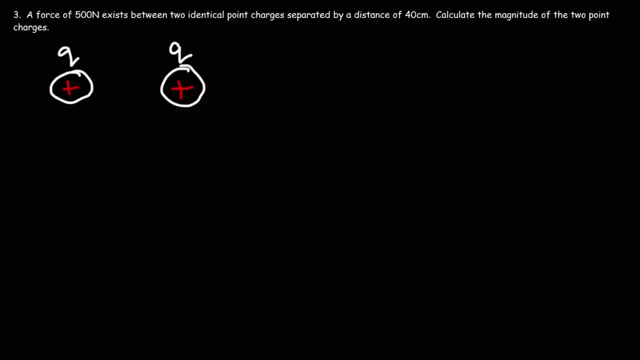 We can simply refer to them as Q, because they're the same, As the problem mentions. they are identical. Now we know the distance between the two point charges, And so that is our R value, which is 40 centimeters. Now we want to convert that to meters. 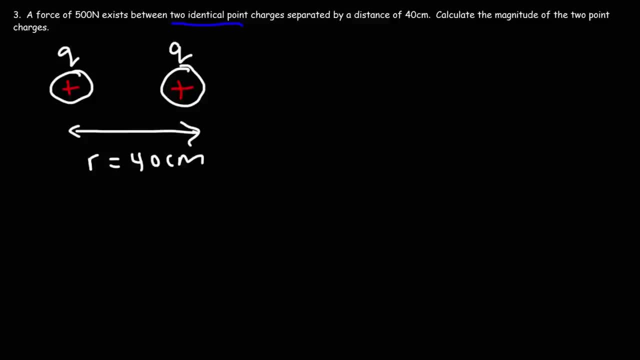 So to quickly convert centimeters to meters, simply divide by 100 or move the decimal two units to the left. So 40 centimeters is equivalent to 0.40 or 0.4 meters. Now we have the magnitude of the force that repels these two charges away from each other. 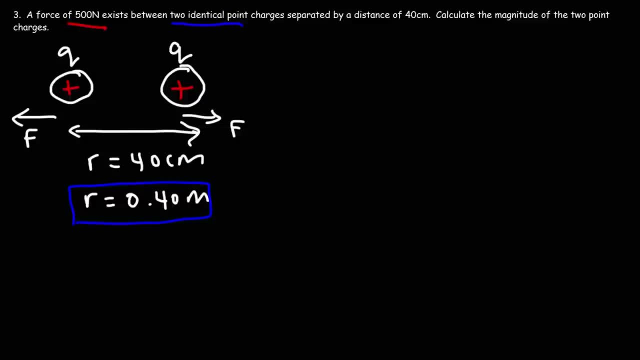 That's 500 newtons. How can we calculate Q? Well, let's begin by writing the formula: F is equal to K. Now, typically we would write Q1 and Q2.. But we're going to replace Q1 with Q and Q2 with Q. 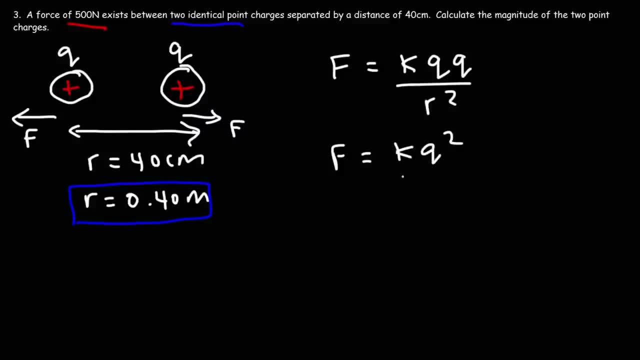 So Q times Q is Q squared. Now what we need to do is we need to isolate Q squared. So I'm going to multiply both sides by R squared over K. The reason why I want to multiply both sides of the equation by R squared over K is so that on the right, we could cancel R squared and we can also cancel K. 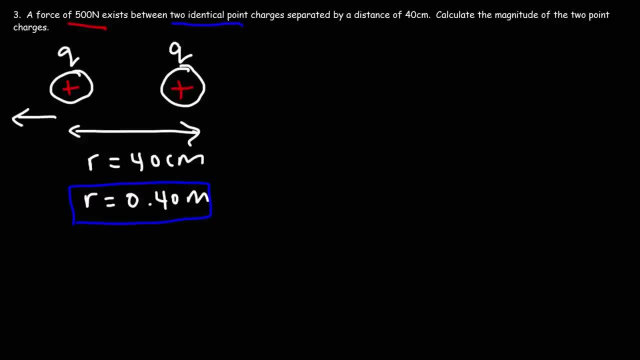 magnitude of the force that repels these two charges away from each other, that's 500 units. how can we calculate Q? well, let's begin by writing: the formula F is equal to K. now, typically we would write Q 1 and Q 2, but we're going to replace Q 1 with Q and Q 2 with Q. so Q times Q is Q squared. 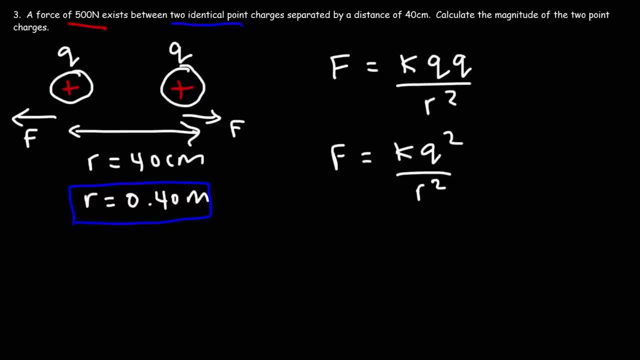 now what we need to do is we need to isolate Q squared, so I'm going to multiply both sides by R squared over K. the reason why I want to multiply both sides of the equation by R squared over K is so that on the right we could 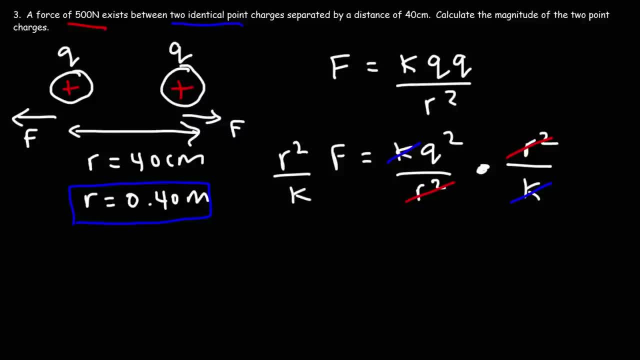 cancel R squared over K so that we could cancel R squared over K. so R squared and we can also cancel K. so what we have left over on the right side, which is now on the left side because I reversed it, is Q squared. Q squared is equal to F times R squared over K. now to get Q, we need to take the. 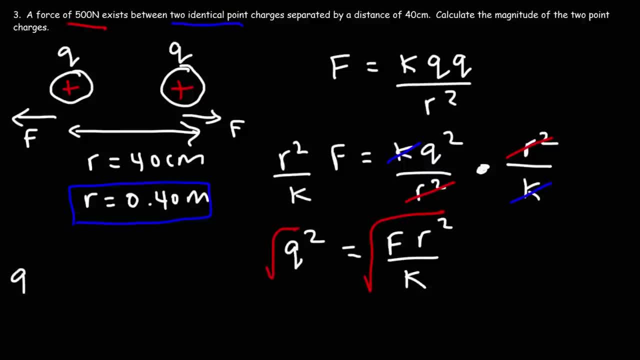 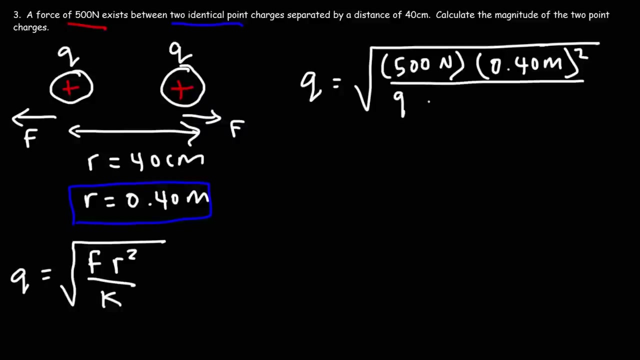 square root of both sides. so for this particular problem, because the two charges are identical, we can calculate Q using this formula. it's going to be equal: the force times the square of the distance divided by K. So the force is 500 Newtons, R is 0.4 meters, and then K is 9 times 10 to the 9, with the. 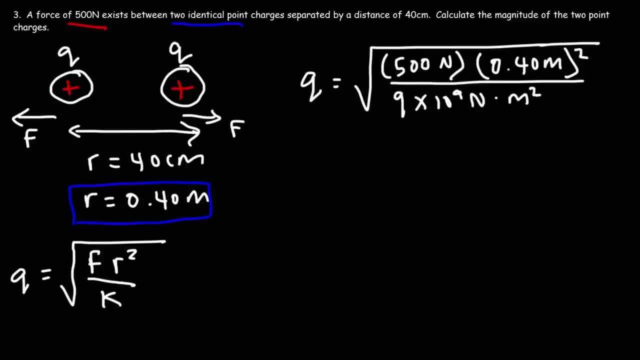 units Newtons times square meters over square coulombs. So we can see the unit Newtons will cancel and the unit square meters will cancel, And so we're going to be left behind with square coulombs. but when we take the square, 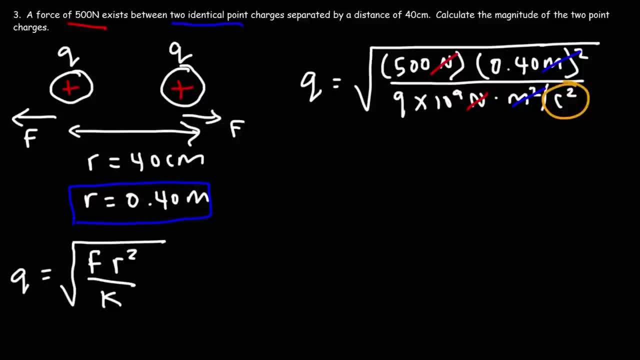 root of that. the unit will just be in coulombs, So let's go ahead and plug this in. So it's the square root of 500 times 0.4, squared, divided by 9 times 10 to the 9, all within. 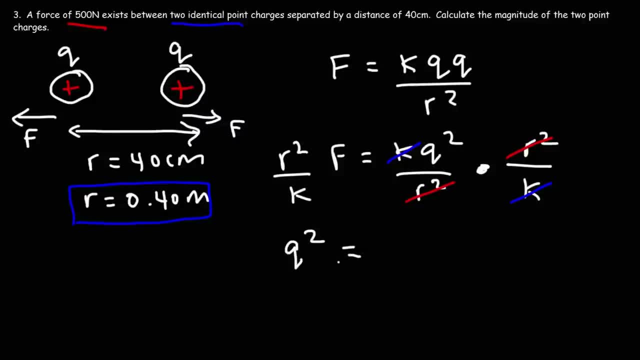 So what we have left over on the right side, which is now on the left side because I reversed it, is Q squared. Q squared is equal to F times R squared over K. Now to get Q, we need to take the square root of both sides. 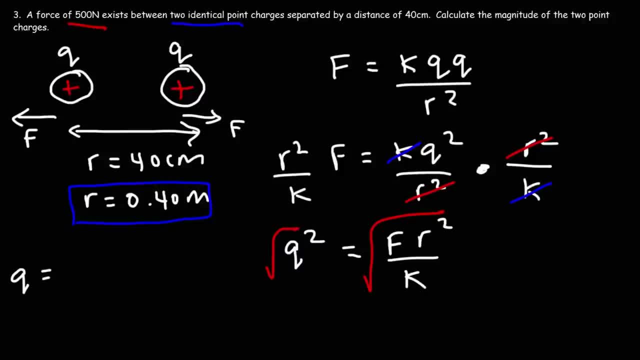 So for this particular problem, because the two charges are identical, we can calculate Q using this formula: It's going to be equal to the force times the square of the distance divided by K. So the force is 500 newtons, R is 0.5.. 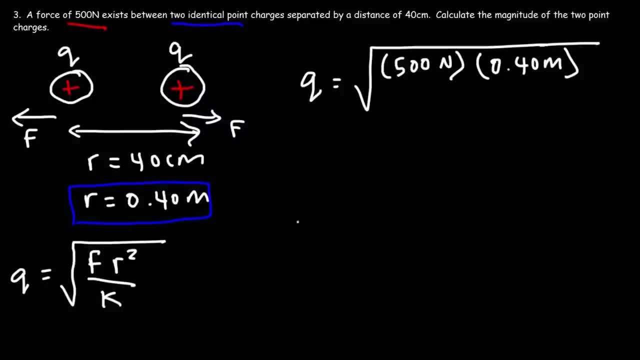 4 meters And then K is 9 times 10 to the 9 with the units newtons times square meters over square coulombs. So we can see the unit newtons will cancel and the unit square meters will cancel, And so we're going to be left behind with square coulombs. 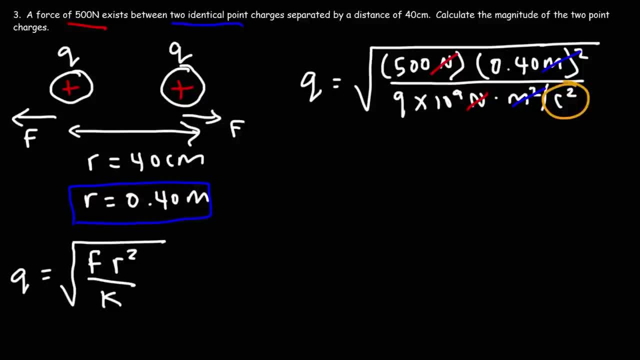 But when we take the square root of that, the unit will just be infinite. So let's go ahead and plug this in. So it's the square root of 500 times 0.4, squared, divided by 9 times 10 to the 9, all within the square root symbol. 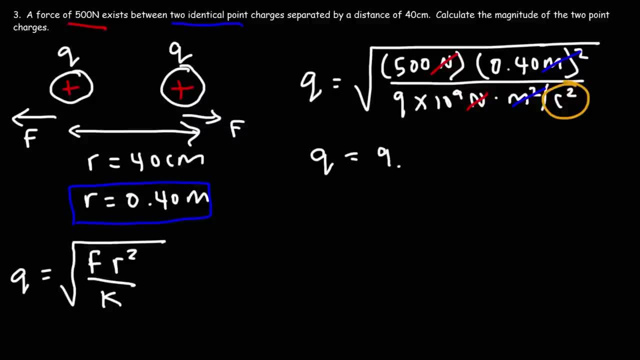 So you should get 9.428 times 10 to the negative 5 coulombs. Now to get the answer in microcoulombs, I'm going to take the square root of 500 times 0.4 squared. Take this value and divide it by 10 to the negative 6, or 1 times 10 to the minus 6.. 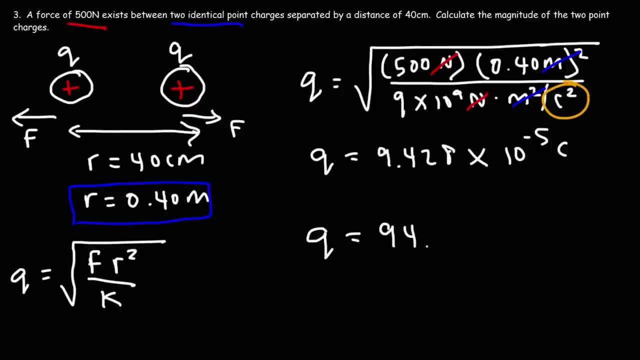 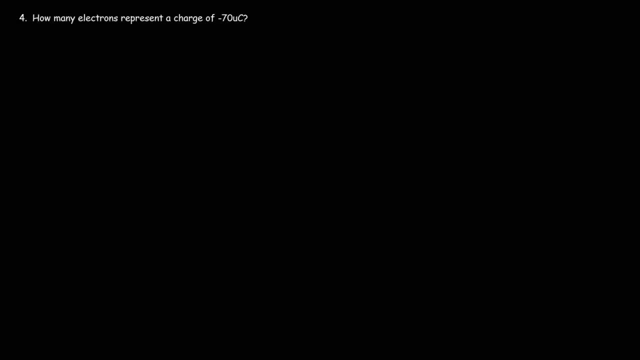 So if you do that, you should get 94.28 microcouplems. So that is the magnitude of the two identical charges. Now let's move on to number 4.. Number 4. How many electrons represent a charge of negative 70 microcouplems? 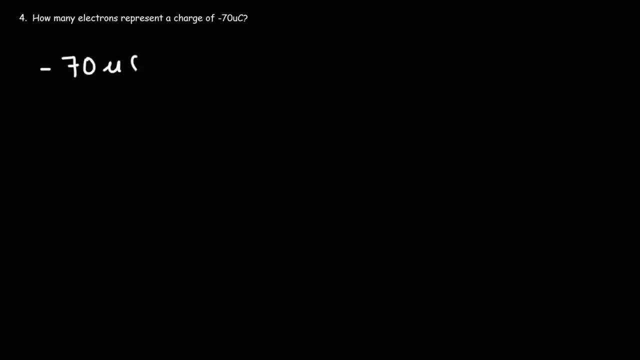 What we can do is we can convert this to the number of electrons. First let's convert it to coulombs. We know 1 microcouplem is 1 times 10 to the negative 6 coulombs. So we can cancel the unit microcouplems. 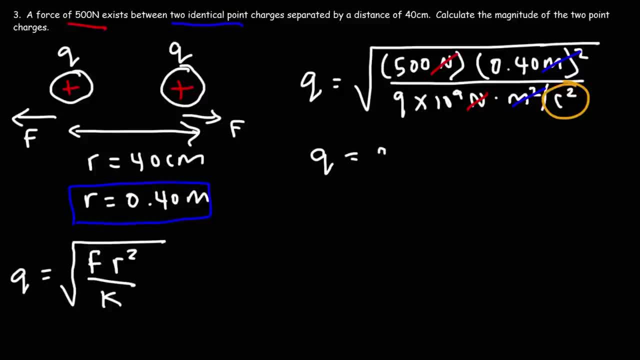 the square root symbol. So you should get 9.428 times 10 to the 9. That's 10 to the negative, 5 coulombs. Now to get the answer in microcoulombs, take this value and divide it by 10 to the negative. 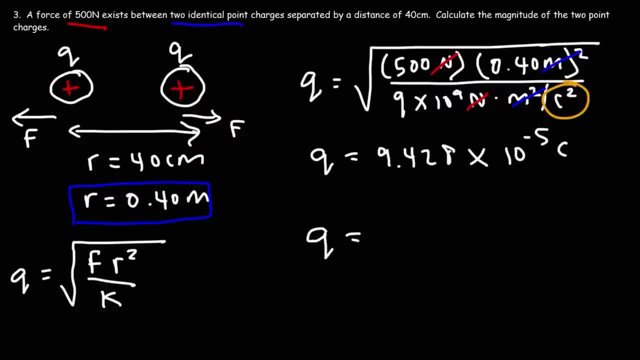 6, or 1 times 10 to the minus 6.. So if you do that you should get 94.28 microcoulombs. So that is the magnitude of the two identical charges. So that is the magnitude of the two identical charges. 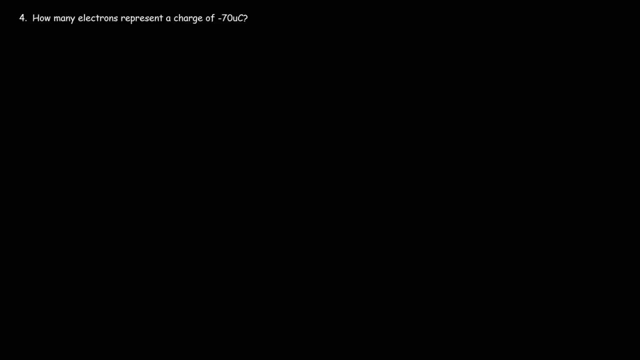 So that is the magnitude of the two identical charges. Now let's move on to number four. How many electrons represent a charge of negative 70 microcoulombs? What we can do is we can convert this to the number of electrons. First, let's convert it to coulombs. 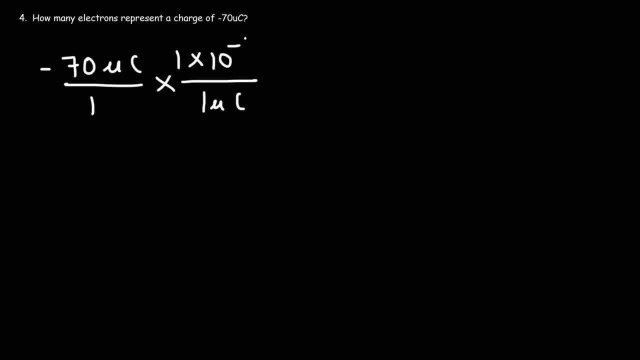 We know 1 microcoulomb is 1 times 10 to the negative 6 coulombs, So we can cancel the unit microcoulombs. What's the conversion factor between number of electrons and electric charge? Keep in mind: 1 electron has an electric charge of negative 1.6 times 10 to the negative 19. 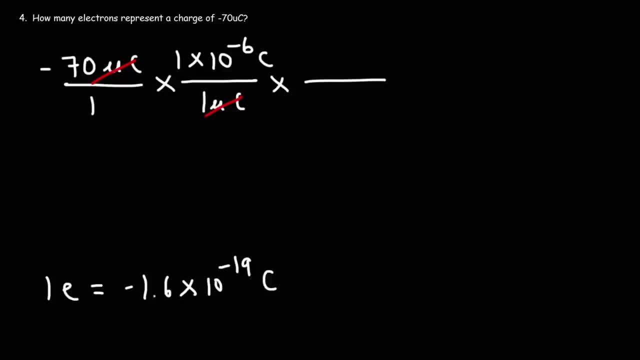 coulombs It's really negative 1.602, but if you round it to negative 1.6, your answer will still be accurate. So let's put coulombs on the bottom and then 1 electron on top. 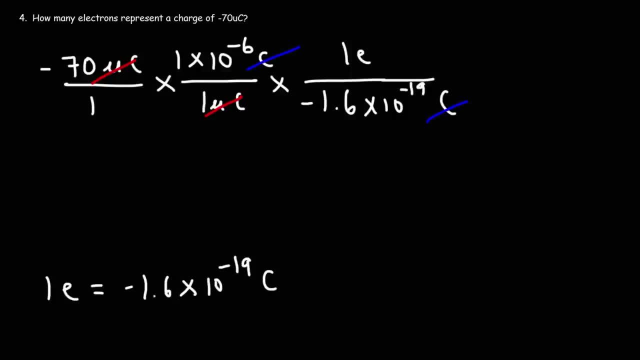 So now we can cancel the unit coulombs. So it's going to be negative 70 microcoulombs times 1 times 10 to negative 6, divided by negative 1.6 times 10 to negative 19.. So the answer is 4.375 times 10 to the 14 electrons. So that's how. 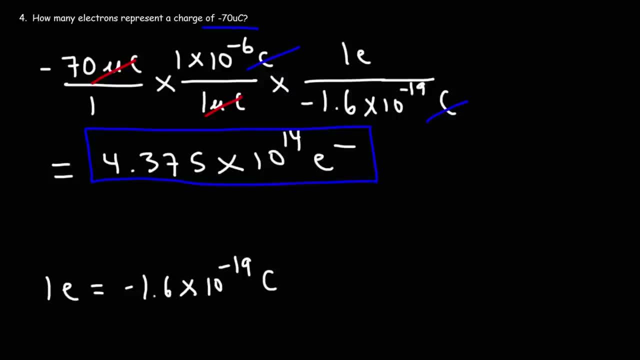 many electrons are represented by a charge of negative 70 microclumes. Now what about number 5? What is the electric charge in microclumes of 5 times 10 to the 14 protons? So for this problem we're going backwards, We're. 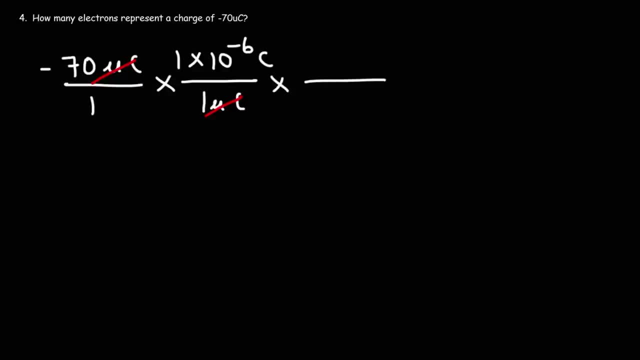 Now we have the conversion factor between the number of electrons and the electric charge. Keep in mind: 1 electron has an electric charge of negative 1.6 times 10. to the negative 19 coulombs It's really negative 1.602, but if you round it to negative 1.6,. 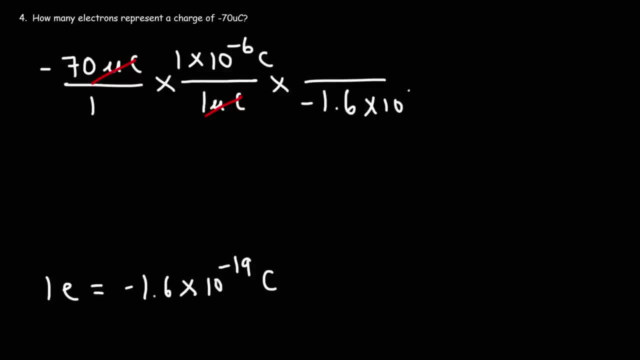 your answer will still be accurate. So let's put coulombs on the bottom and then 1 electron on top, So now we can cancel the unit coulombs. So it's going to be negative 70 times, 1 times 10 to the negative 70,. 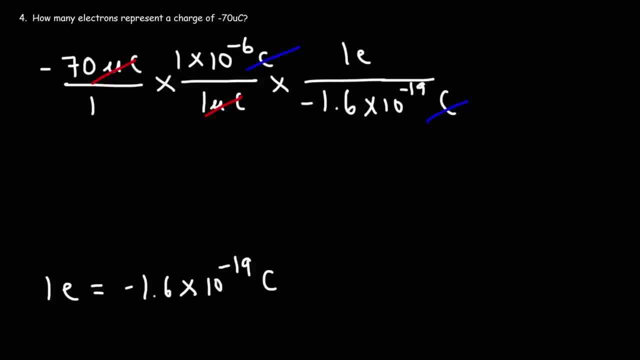 divided by negative, 1.6 times 10 to the negative 19.. So the answer is 4.375 times 10 to the 14 electrons. So that's how many electrons are represented by a charge of negative 70 microcouplems. 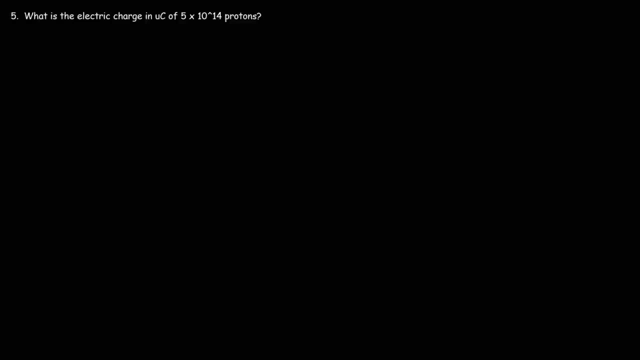 Now what about number 5?? What is the electric charge in microcouplems? What is the electric charge in microcouplems? So for this problem we're going backwards, We're converting number of protons to electric charge. So let's start with what we're given 5 times 10 to the 14 protons. 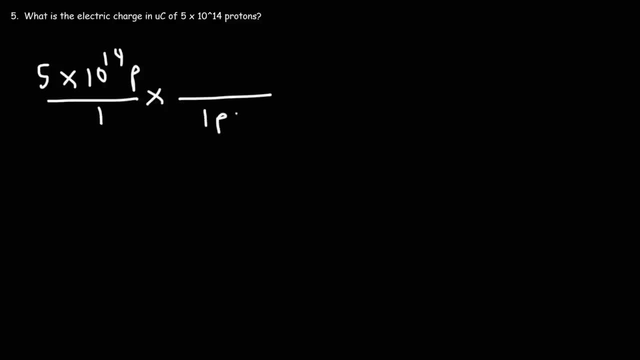 Now let's convert protons to charge. We know that 1 proton has a charge of positive 1.6 times 10 to the 19 coulombs And we know that 7 times 10 to the 19 coulombs is positive 1.6 times 10 to the 19 coulombs. 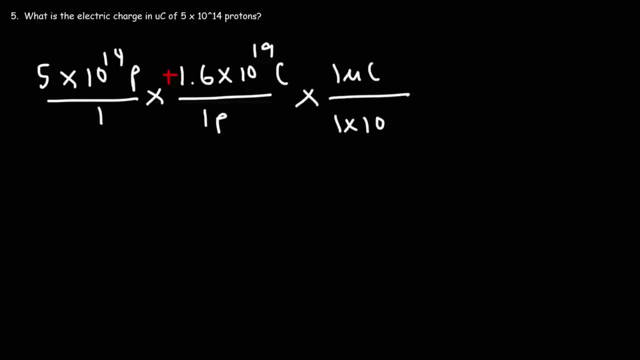 one microclume is 1 times 10 to the negative 6 columns. so the number of protons cancels and the charging columns cancel, so we get to charge in micro columns. so it's going to be- oh, by the way, this is negative- 19, so it's 5 times. 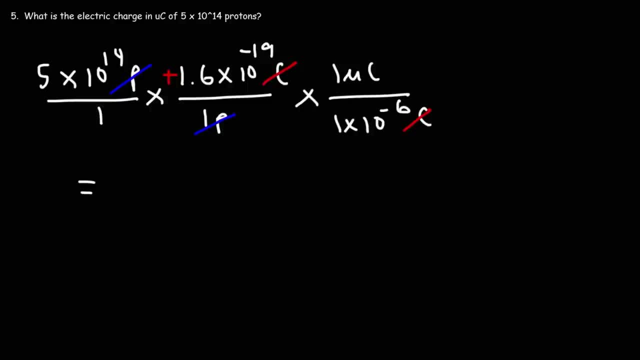 10 to the 14 times 1.6 times 10 to negative 19, and then take that result divided by 1 times 10 to negative 6 and you should get 80. so the charge that it represents is positive 80 microclumes. so that's the answer for number 5. number 6: 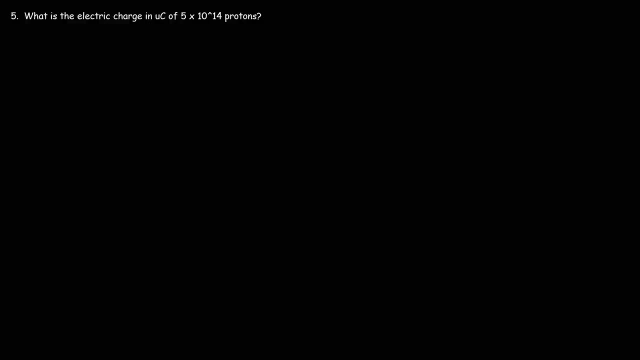 converting number of protons to electric charge. So let's start with what we're given, 5 times 10 to the 14 protons. Now let's convert protons to charge. We know that one proton has a charge of positive 1.6. 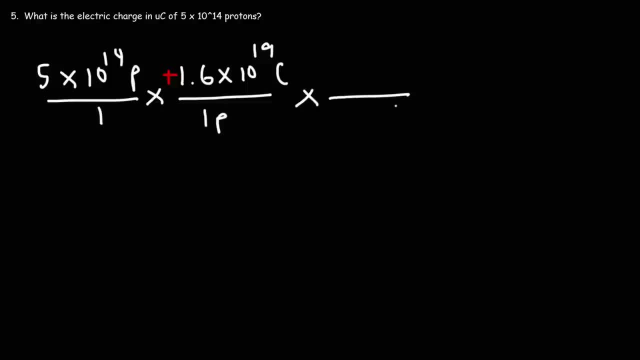 times 10 to the 19 clumes. And we know that one microclume is 1 times 10 to the negative 6 clumes. So the number of protons cancels and the charge in clumes cancel, So we get the charge in microclumes. So it's going to be oh by. 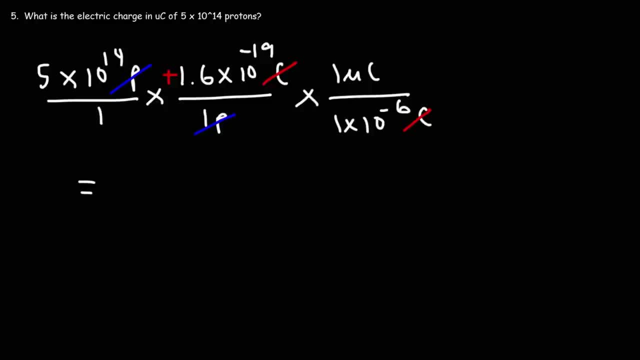 the way this is negative 19.. So it's 5 times 10 to the 14 times 1.6 times 10 to negative 19.. And then take that result divided by 1 times 10 to the negative 6. And you should: 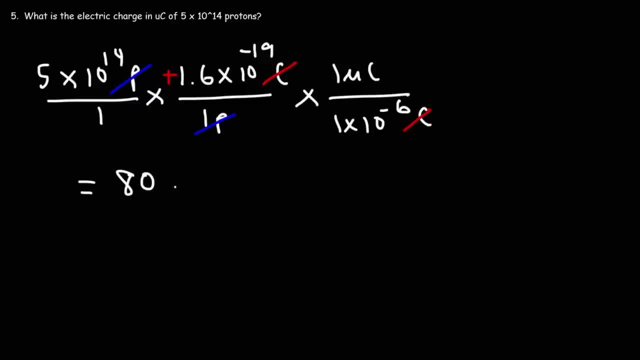 get 80.. So the charge that it represents is positive 80 microclumes. So that's the answer for number 5.. Number 6,: a metal sphere has 4.3 times 10 to the 21 protons and 6.8 times 10 to the 21 electrons. 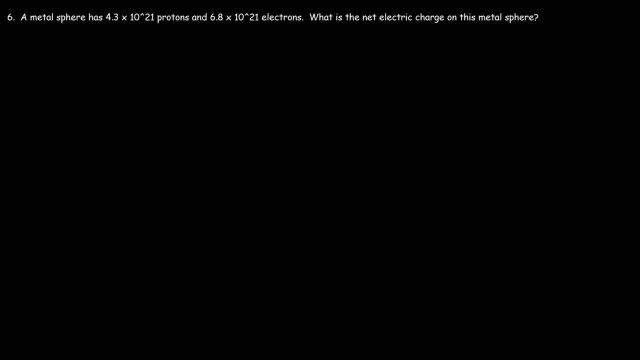 What is the net electric charge on this metal sphere? In order to determine the net electric charge, we need to know if we have more protons than electrons or vice versa. In this case, we have more electrons. What we really need to do is determine the excess number of electrons. 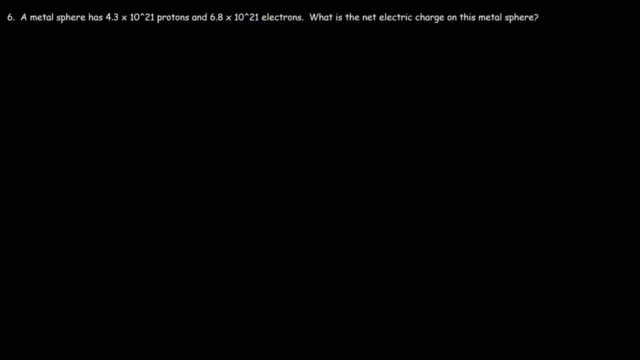 and convert that to electric charge. But there's a simple formula that you could use to get this answer quickly. So the net charge q- let me draw that better- is going to be the difference between the number of protons and electrons. So if we get more protons than electrons, this number- 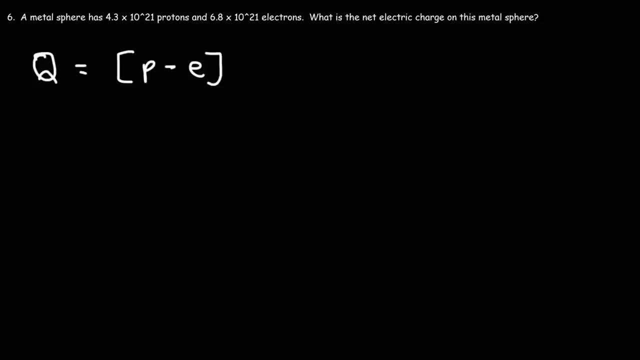 will be positive. If the number of electrons exceeds the protons, this number will be negative. So it's going to be p minus e times the charge of a proton, which is 1.6 times 10, to the negative 19.. 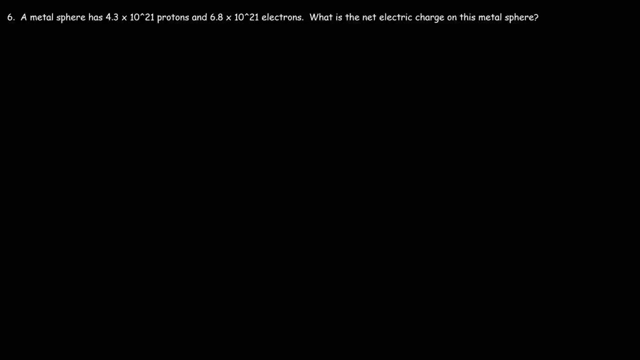 a metal sphere has 4.3 times 10 to the 21 protons and 6.8 times 10 to the 21 electrons. what is the net electric charge on this metal sphere? in order to determine the net electric charge, we need to know if we have more protons than electrons or. 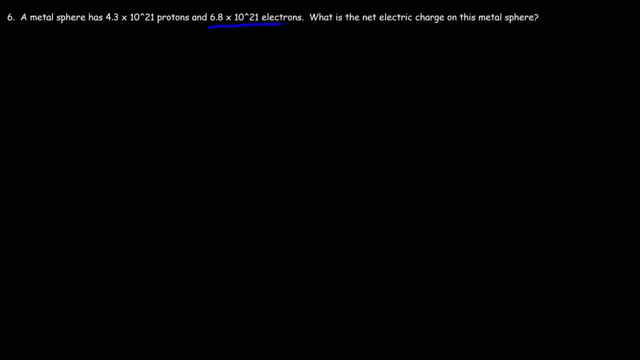 vice-versa. in this case we have more electrons. what we really need to do is determine the excess number of electrons and convert that to electric charge. but there's a simple formula that you could use to get this answer quickly. so So the net charge Q- let me draw that better- is going to be the difference between the 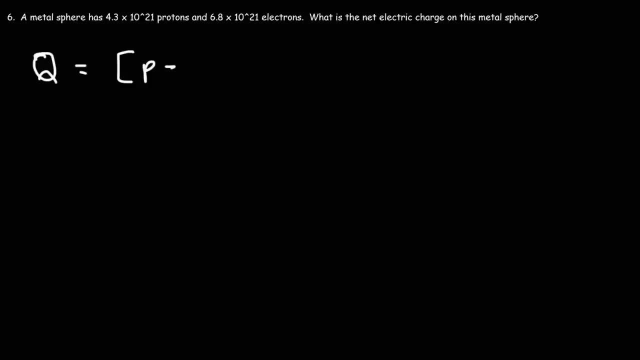 number of protons and electrons. So if we get more protons than electrons, this number will be positive. If the number of electrons exceeds the protons, this number will be negative. So it's going to be P minus E times the charge of a proton, which is 1.6 times 10 to the 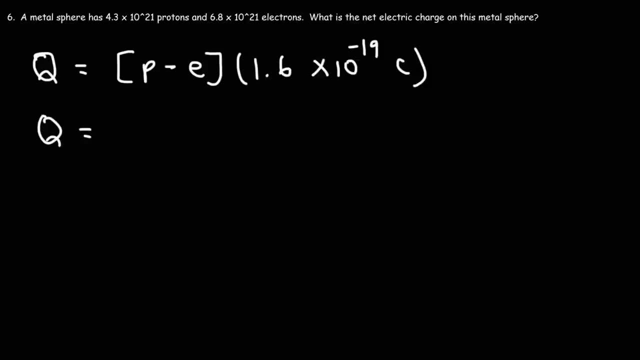 negative 19 coulombs. So for this problem all we need to do is plug in these values. So we have 4.3 times 10 to the 21 protons and we have 6.8 times 10 to the 21 electrons. 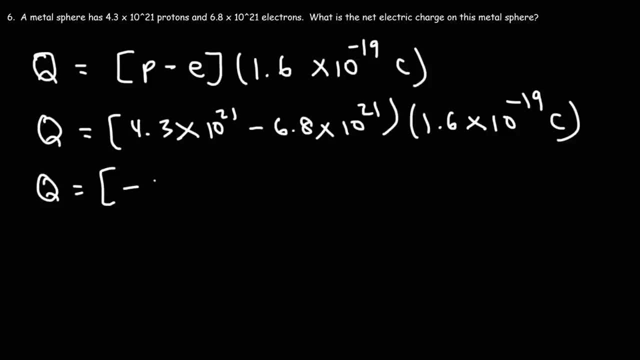 So 4.3 minus 6.8, that's the difference of negative 2.5.. So because it's negative, that tells us that the overall charge will be negative, and so that means that we have more electrons than protons. 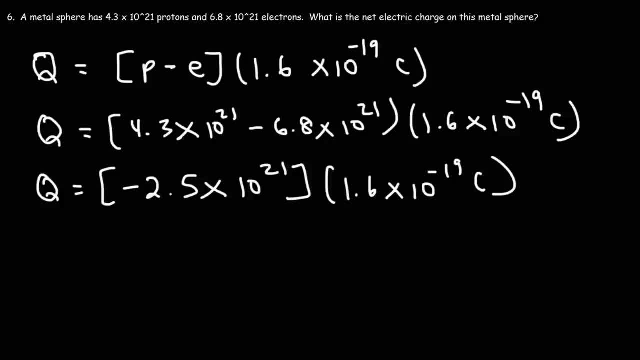 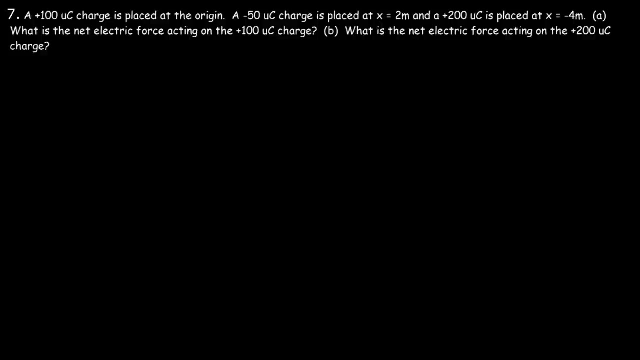 So negative 2.5 times 10 to the 21, times 1.6 times 10 to the negative 19.. This is equal to negative 400 coulombs. That is the net electric charge on this particular metal sphere. A 100 microcoulomb charge is placed at the origin. 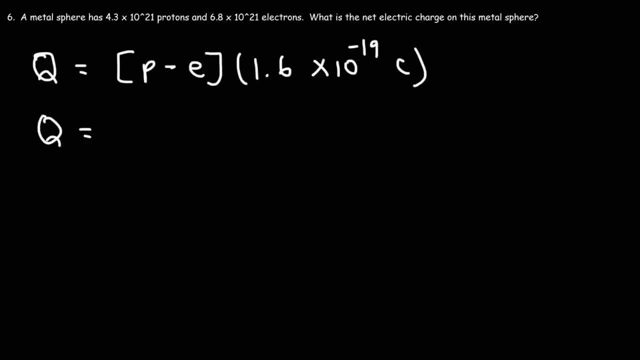 Clumes this problem. all we need to do is plug in these values. so we have 4.3 times 10 to 21 protons and we have 6.8 times 10 to 21 electrons. so 4.3 minus 6.8, that's. 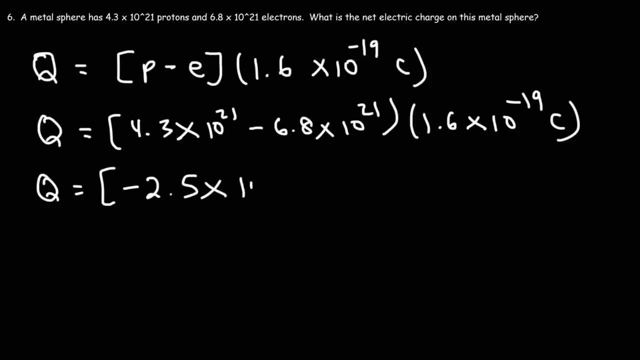 the difference of negative 2.5. so because it's negative, that tells us that the overall charge will be negative and so that means that we have more electrons and protons. so negative 2.5 times 10 to 21 times 1.6 times 10 to the negative 19, this is: 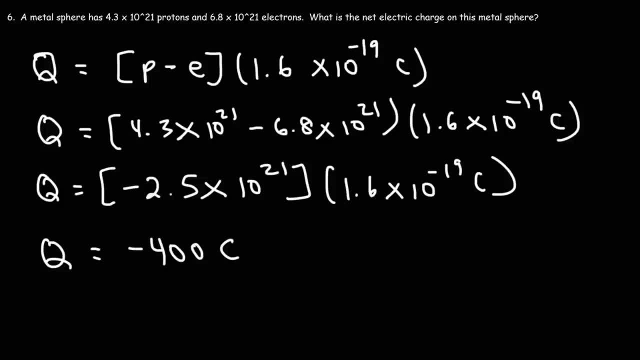 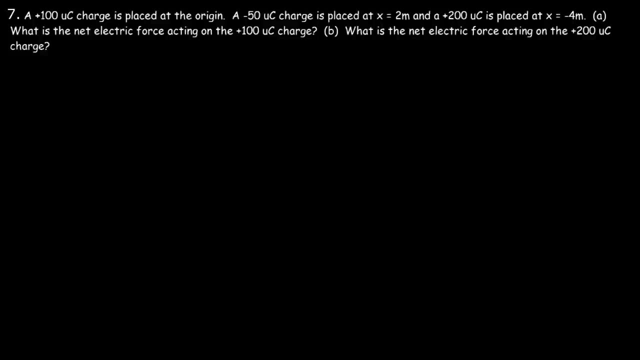 equal to negative 400 coulombs, so that is the net electric charge on this particular metal sphere. a 100 microcoulomb charge is placed at the origin. a negative 50 microcoulomb charge is placed at x equals 2 meters relative to the origin and a 200 microcoulomb 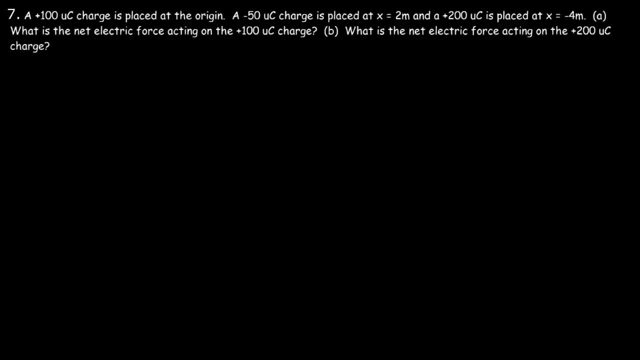 charge is placed at x equals negative 4 meters. what is the net electric force acting on the 100 microcoulomb charge? so if you want to try this problem, feel free and pause the video to see if you can get the right answer. so go ahead and work on this problem now. the first thing we need to do is draw a. 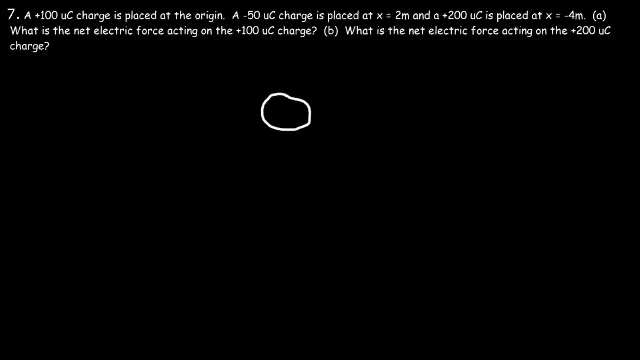 picture. so we have a positive charge placed at the origin, and that's the 100 microclume charge, and then, at a position of 2 meters relative to the origin, we have a negative charge with a magnitude of negative 50 microclumes, and then on. 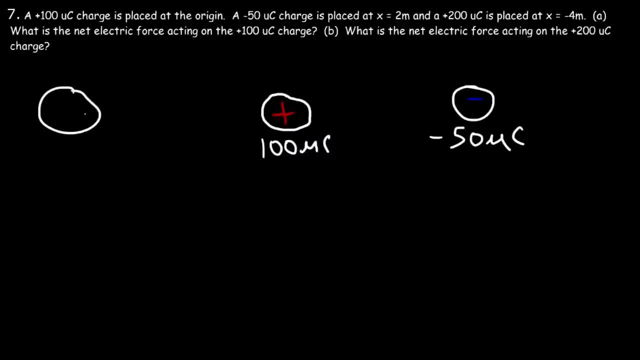 the left side, at negative 4 meters, we have a positive charge with a magnitude of 200 microclumes. so the distance between these two charges is 4 meters and between the two charges on the right it's 2 meters. let's call this q1, q2 and. 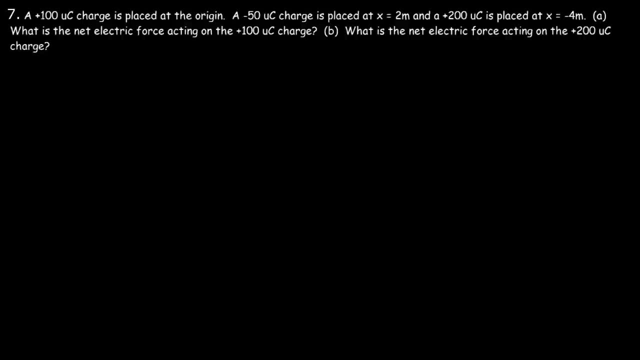 A negative 50 microcoulomb charge is placed at x equals 2 meters relative to the origin, and a 200 microcoulomb charge is placed at x equals negative 4 meters. What is the net electric force acting on the 100 microcoulomb charge? 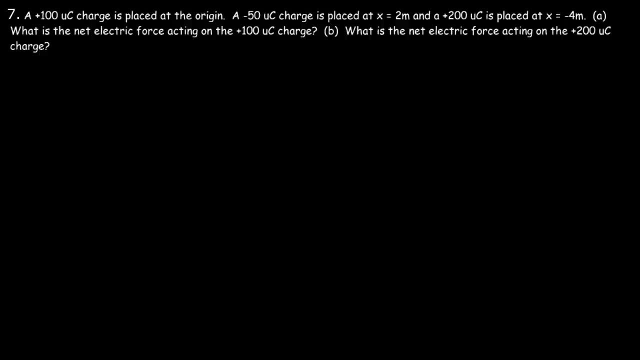 So if you want to try this problem, feel free And pause the video to see if you can get the right answer. So go ahead and work on this problem Now. the first thing we need to do is draw a picture, So we have a positive charge placed at the origin, and that's the 100 microcoulomb charge. 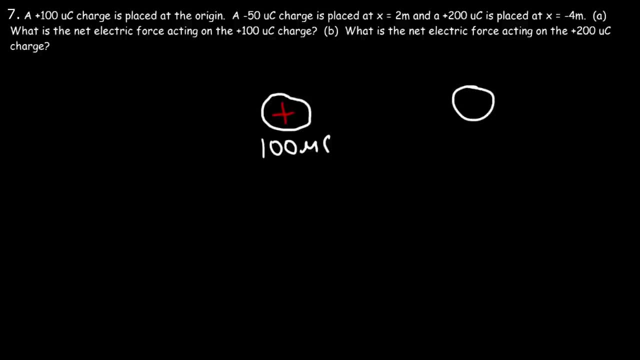 And then, at a position of 2 meters relative to the origin, we have a negative charge with a magnitude of negative 50 microcoulombs. And then, on the left side, at x equals 2 meters relative to the origin, we have a negative charge with a magnitude of negative 50 microcoulombs. 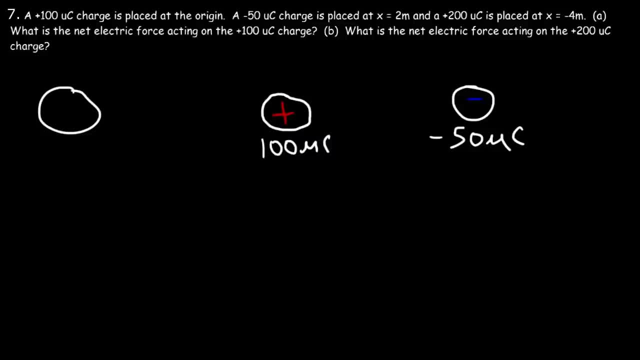 And then, at a position of negative 4 meters, we have a positive charge with a magnitude of 200 microcoulombs. So the distance between these two charges is 4 meters and between the two charges on the right it's 2 meters. 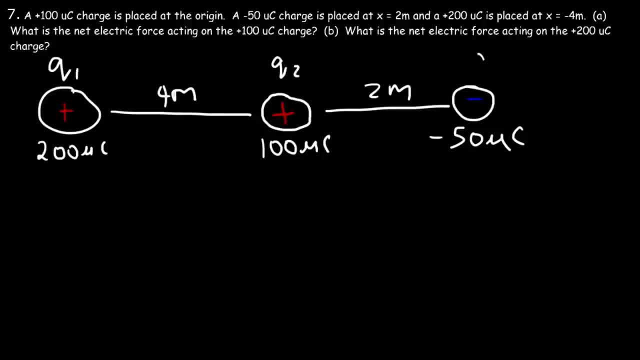 Let's call this Q1,, Q2, and Q3.. So how can we use this information to determine the net electric force acting on the middle charge? First we'll need to identify all the forces acting on the middle charge. So Q2 fills a force of attraction with Q3.. 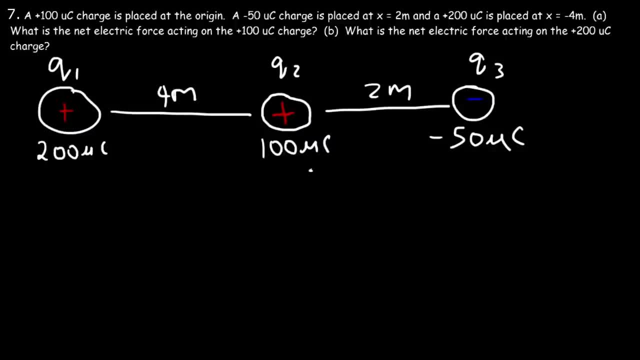 Q2 is attracted to Q3. So there's going to be a force that's going to accelerate Q2 towards Q3. And we're going to call that force F2,3.. So this is the force on 2 due to charge 3.. 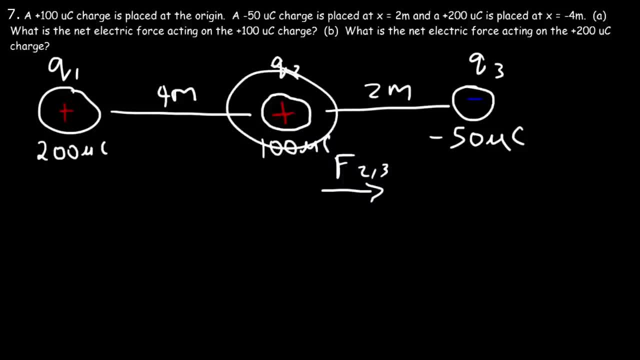 Now Q2,, with its positive charge, is repelled by Q1. So Q2 wants to move away from Q1.. So there's another force acting on Q2, and that's going to be F2,1.. That is the force acting on charge 2 due to charge 1.. 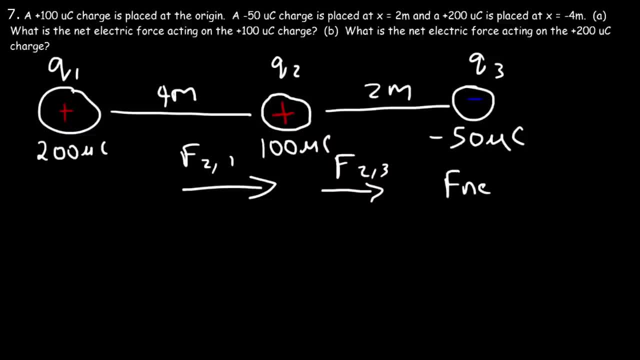 And so the net force is going to be the sum of these two forces. Anytime you have two vectors that are parallel to each other, to find the sum of those vectors you can simply add them. So the net force is going to be F1 and 2. 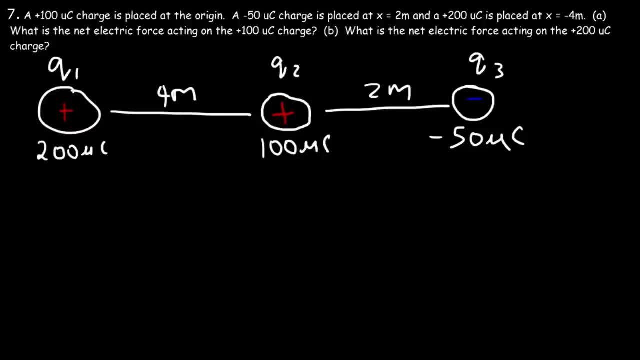 q3. so how can we use this information to determine the net electric force acting on the middle charge? first we need to identify all the forces acting on the middle charge. so q2 feels a force of attraction with q3. q2 is attracted to q3, so there's going to be a force that's going. 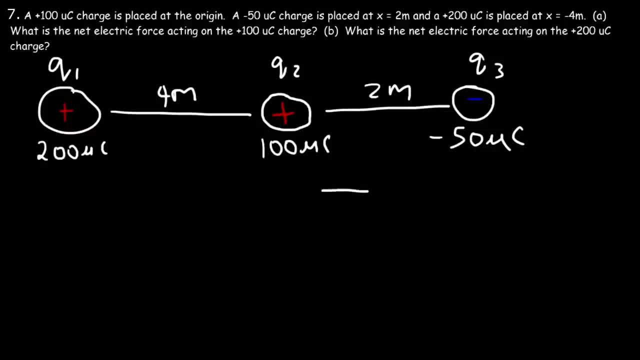 to accelerate q2 towards q3 and we're going to call that force F, 2,, 3.. So this is the force on 2 due to charge 3.. Now Q2,, with its positive charge, is repelled by Q1.. 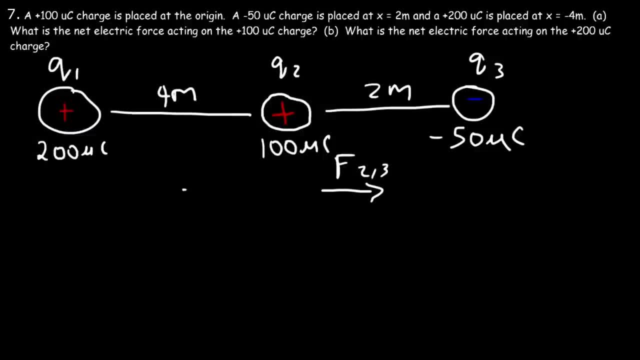 So Q2 wants to move away from Q1.. So there's another force acting on Q2, and that's going to be F 2, 1.. That is the force acting on charge 2 due to charge 1.. And so the net force is going to be the sum of these two forces. 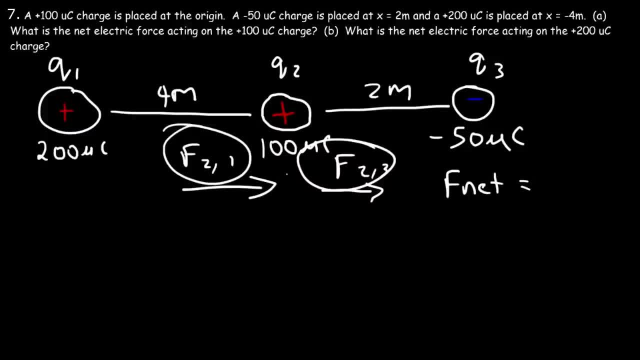 Anytime you have two vectors that are parallel to each other, to find the sum of those vectors you can simply add them. So the net force is going to be F 2 on 1, I mean F 1 on 2, rather. 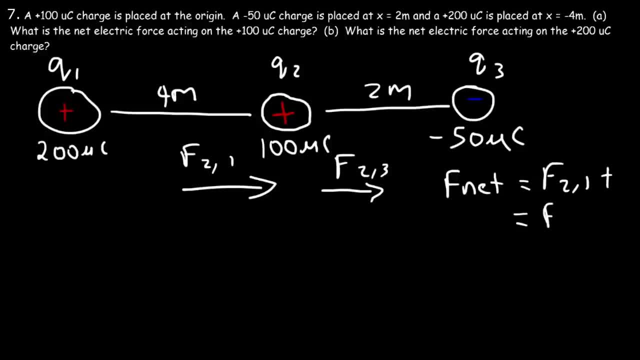 plus F 3 on 2, or the force exerted on 2 by a charge 3.. So we just got to add those two values. So first we need to calculate each one. So let's calculate F 2, 1.. 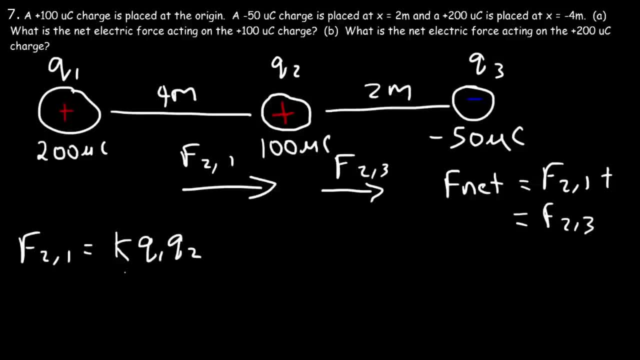 So it's going to be K times Q1 times Q2, divided by R squared, where R is the distance between Q1 and Q2.. So K is 9 times 10 to the 9.. Q1 is 200 microcouple, or 200 times 10 to the minus 6.. 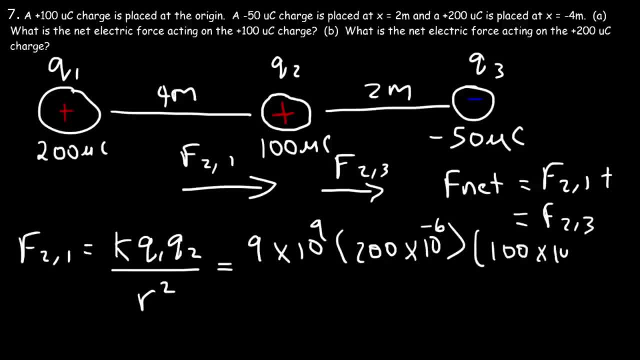 And Q2 is 100 times 10 to the negative. So Q1 is the distance between Q2 and Q6.. Divided by R squared or four squared. So go ahead and type that in. Thank you, End End. 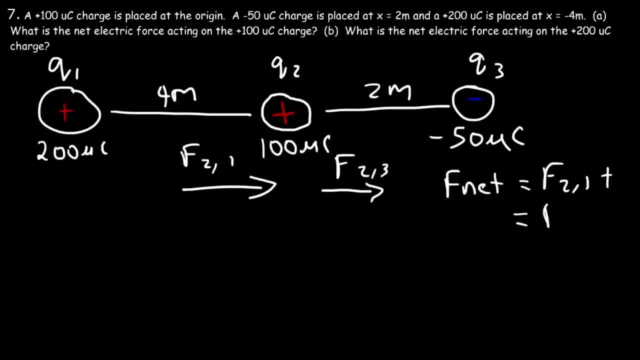 plus F3 on 2, or the force exerted on 2 by a charge 3.. So we've just got to add those two values. So first we need to calculate each one. So let's calculate F2,1.. 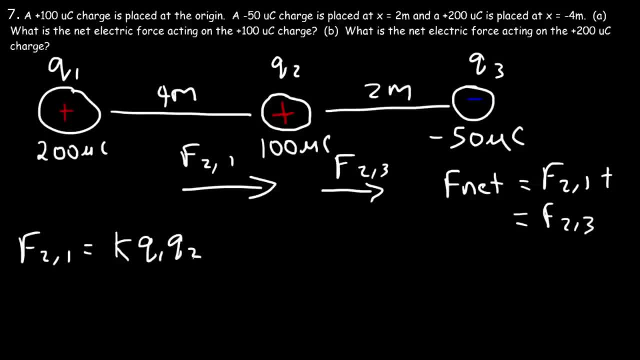 So it's going to be K times Q1 times Q2.. Q2 divided by R, squared, where R is the distance between Q1 and Q2.. So K is 9 times 10 to the 9.. Q1 is 200 microclones, or 200 times 10 to the minus 6.. 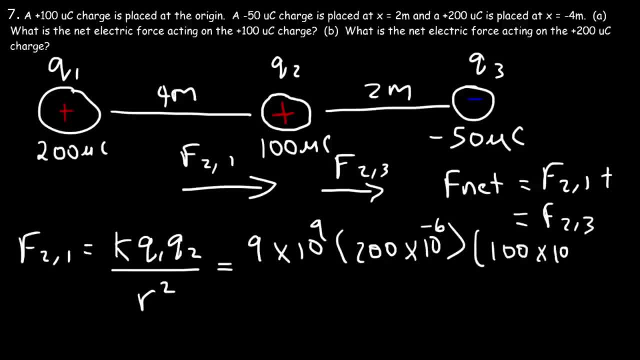 And Q2 is 100 times 10, to the negative 6, divided by R squared or 4 squared. So go ahead and type that in. So the net force is going to be F2,1.. So the force exerted on charge 2 by a charge 1 is 11.25 Newton. 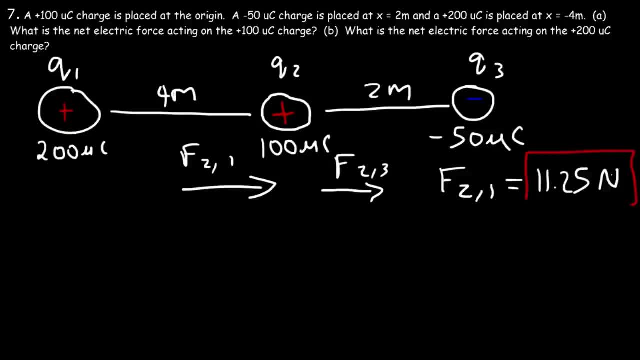 So that's 11.25 Newton. So let's save that answer. We're going to use it later. Now we need to calculate the force exerted on charge 2 by charge 3.. So that's going to be KQ2 times Q3 over R squared. 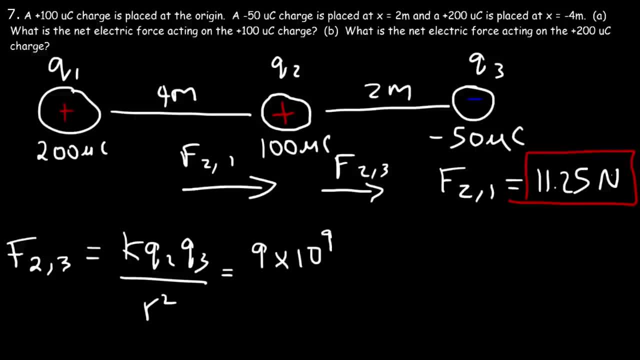 So K is a constant, It's not going to change. It's 9 times 10 to the 9.. Q2 is 100 times 10 to the minus 6.. And Q3 is 50 times 10 to the negative 6.. 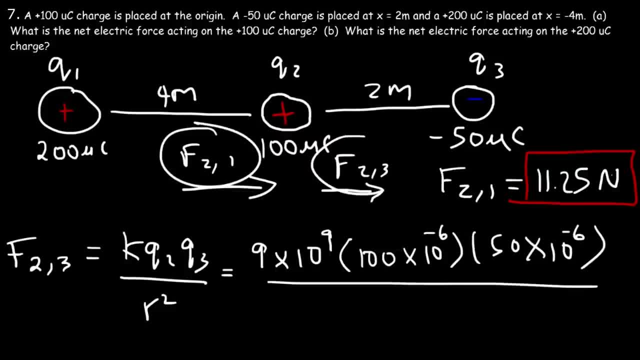 Don't worry about the negative sign. These two forces are positive because they're both directed along the positive X direction, So you can adjust the sign based on the direction of the force. Now R- the distance between Q2 and Q3, is 2 meters. 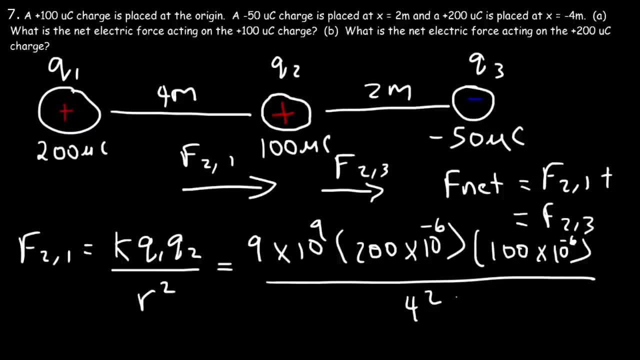 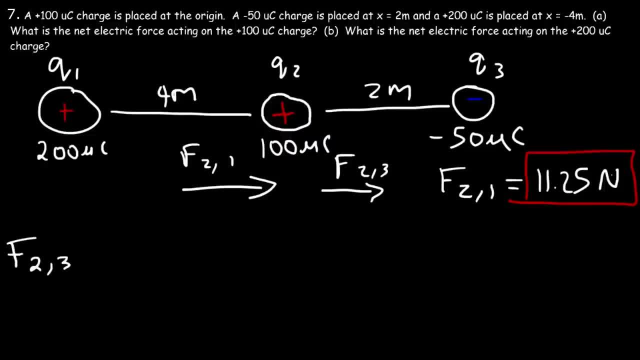 Now we need to calculate the force exerted on charge 2 by charge 3.. So that's going to be K Q2 times Q3 over R squared. So K is a constant, it's not going to change. It's 9 times 10 to the 9, Q2 is 100 times 10 to the minus 6, and Q3 is 50 times 10 to. 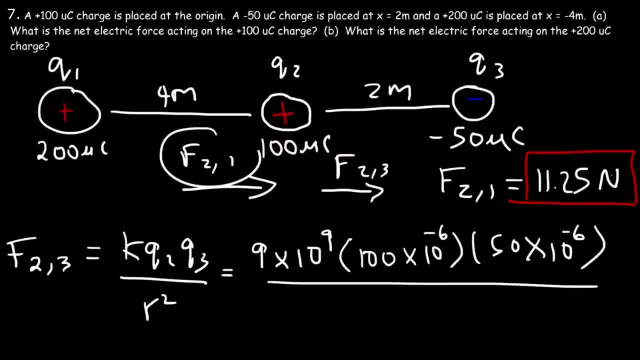 negative 6.. Don't worry about the negative sign. These two forces are positive because they're both directed along the positive X direction, So you can adjust the sign based on the direction of the force. Now R, the distance between Q2 and Q3 is 2 meters. 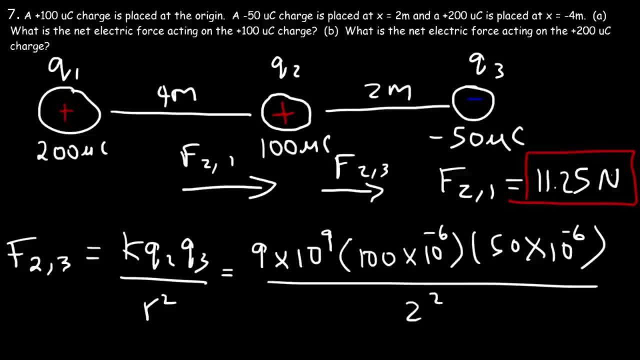 So we're going to divide it by 2 squared. It turns out that F2 comma 3 is equal to the same number, 11.25 Newtons- purely by coincidence. So now we can calculate the net force acting on charge 2.. 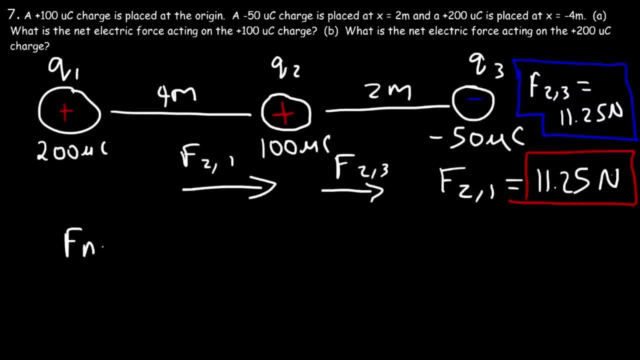 So, as we said before, the net force is simply the sum of these two forces, because they're going in the same direction. So it's F2,1 plus F2,3.. And so that's going to be 11.25 plus 11.25, which adds up to 22.5 Newtons. 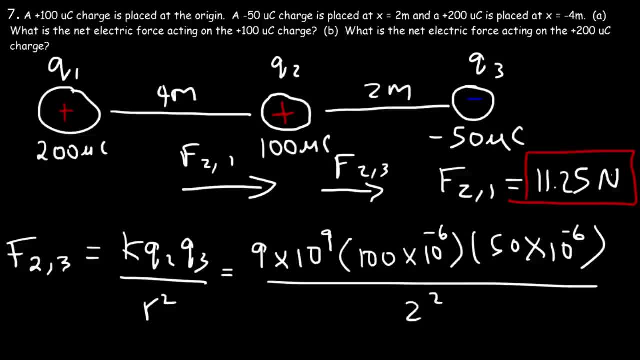 So we're going to divide it by 2 squared, It turns out that F2,3 is equal to the same number, 11.25 newtons, purely by coincidence. So now we can calculate the net force acting on charge 2.. 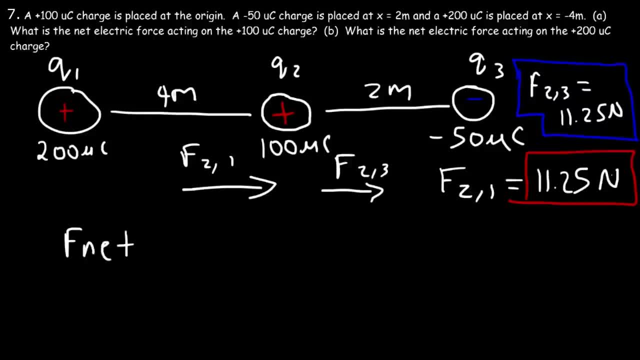 So, as we said before, the net force is simply the sum of these two forces, because they're both directed along the negative X direction, So they're going in the same direction. So it's F2,1 plus F2,3.. 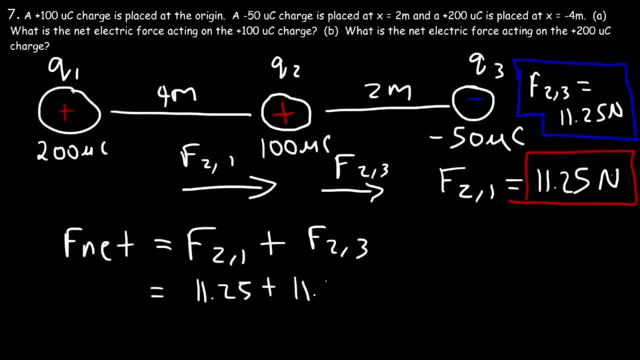 And so that's going to be 11.25 plus 11.25, which adds up to 22.5 newtons. And so that's the answer for part A. Now let's move on to the next part. What is the net electric force acting on the 200 microcoulomb charge? 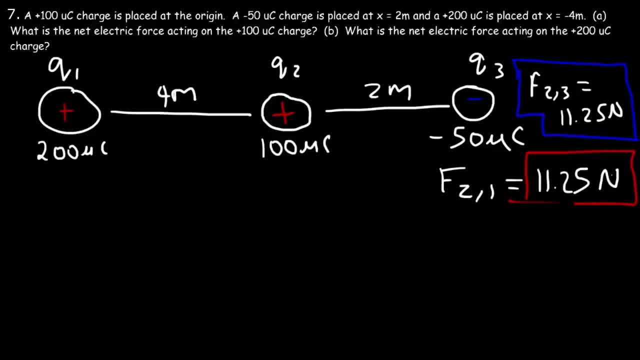 So that's on Q1.. So let's see what effect Q2 has on Q1.. Q2 repels Q1. So Q2 will cause Q1 to go in this direction. So we can call that F, That's the force exerted on charge 1 by charge 2.. 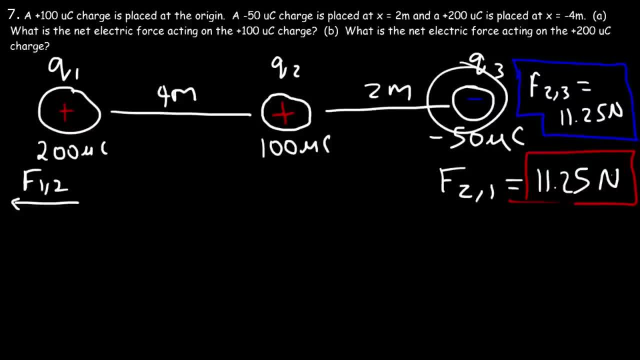 Now Q1 is attracted to Q3, because opposites attract. So we have another force, which we'll call F1,3.. That's the force exerted on charge 1 as a result of charge 3.. Now these two forces are competing with each other. 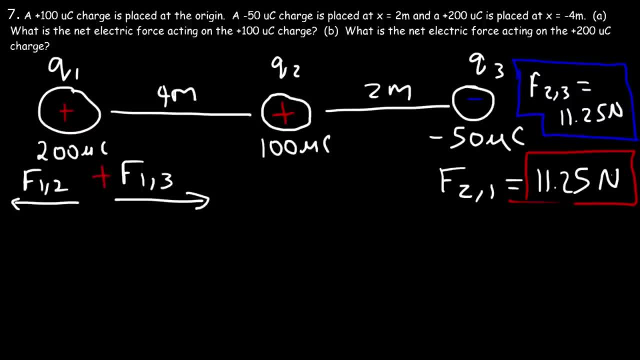 Now. this force is in the positive X direction, so we're going to give it a positive number. This force is in the negative direction, So the net force is going to be the sum of these two values. If the net force is positive, that means that F1,3 is greater, which is probably not because it's so far away. 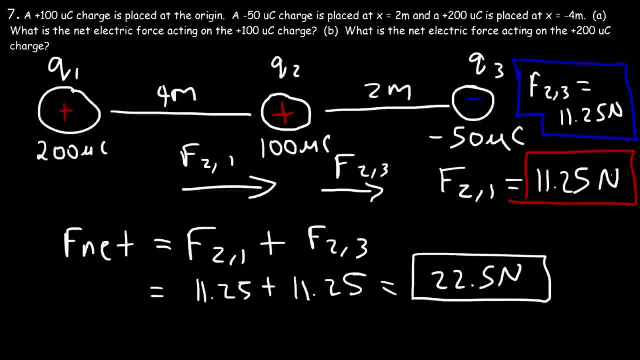 So that's the answer for part A. Now let's move on to the next part. What is the net electric force acting on the 200 microcoulomb charge? So that's on Q1.. So let's see What effect Q2 has on Q1.. 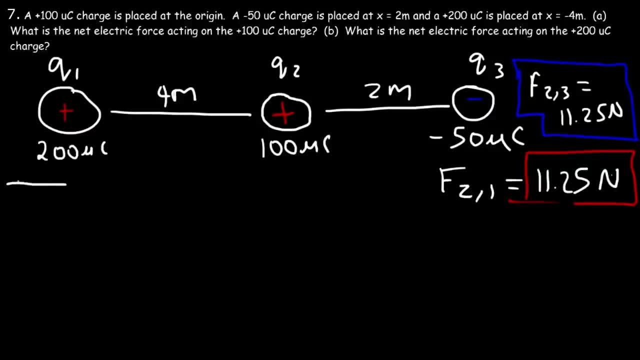 Q2 repels Q1.. So Q2 will cause Q1 to go in this direction, So we can call that F1,2.. That's the force exerted on charge 1 by charge 2.. Now Q1 is attracted to Q3, because opposites attract. 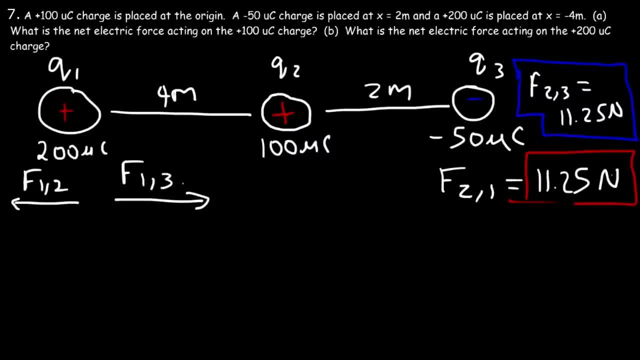 So we have another force, which we'll call F1,3.. That's the force. It's exerted on charge 1 as a result of charge 3.. Now these two forces are competing with each other. Now this force is in a positive X direction. 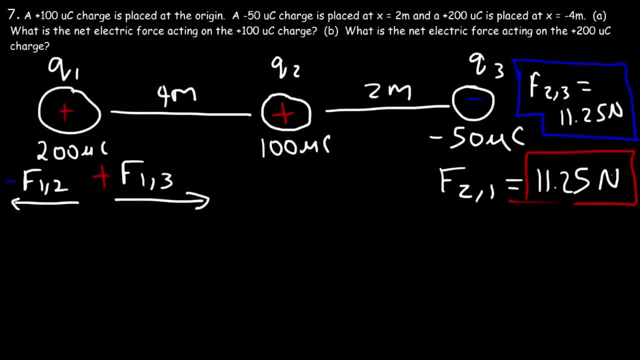 So we're going to give it a positive number. This force is in a negative direction, So the net force is going to be the sum of these two values. If the net force is positive, that means that F1,2,3 is greater, which is probably not because 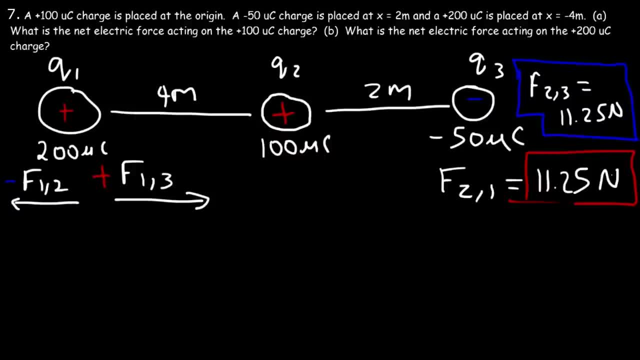 it's so far away. If the net force is negative, which is probably going to be the case, So the net force is negative, That means that this force is greater. So let's calculate the values of each of these two forces. Now it's important to understand that F1,2 is equal to F2,1 in magnitude. 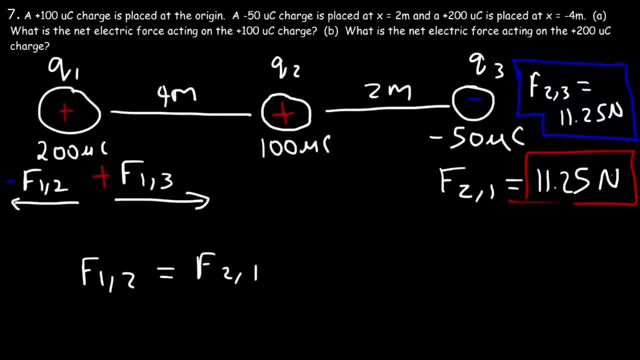 They have the same magnitude, but the direction may not be the same, So the sign might be different. So technically we should say that the absolute value of F1,2 is negative. So the absolute value of F1,2 is negative. 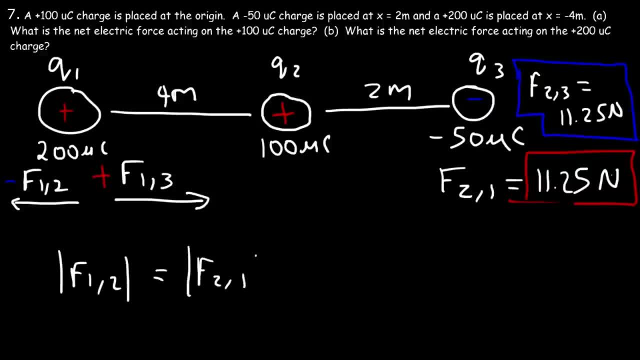 So the absolute value of F1,2 is negative. So the absolute value of F1,2 is equal to the absolute value of F2,1, because one might be negative and the other might be positive. So we don't need to calculate this value because we already have it here. 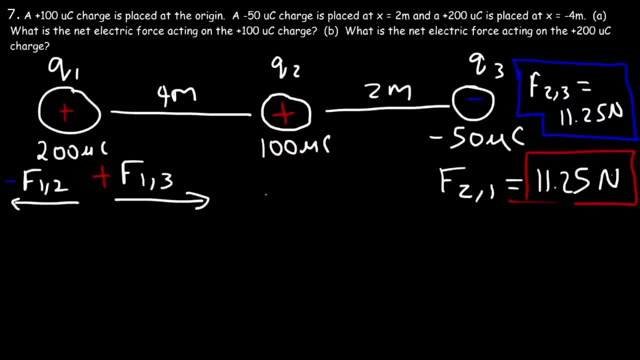 If the net force is negative, which is probably going to be the case, that means that this force is greater. So let's calculate the values of each of these two forces. Now, it's important to understand that F1,2 is equal to F2,1 in magnitude. 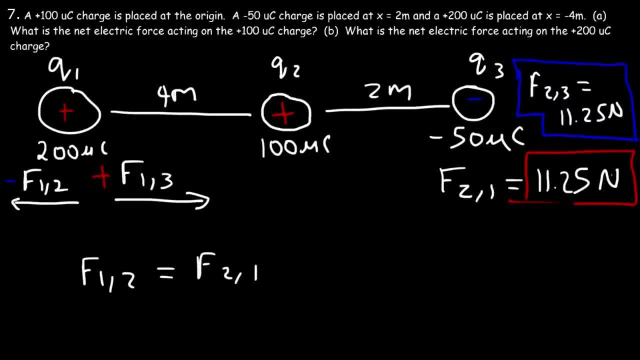 They have the same magnitude but the direction may not be the same, So the sign might be different. So technically we should say that the absolute value of F1,2 is equal to the absolute value of F2,1. Because one might be negative and the other might be positive. 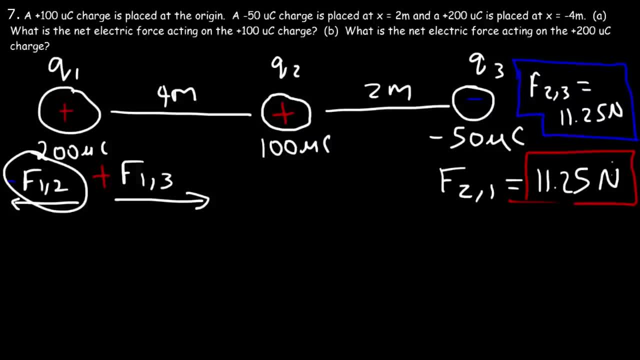 So we don't need to calculate this value because we already have it here. We do, however, need to calculate this value Because we don't have that yet. So F1,3, that's going to equal KQ1Q3 divided by R squared. 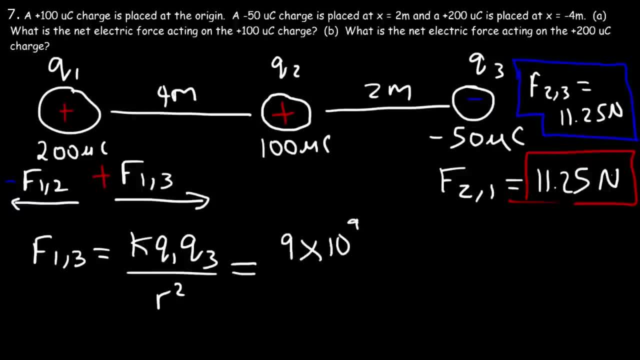 Now K is 9 times 10 to the 9. Q1 is 200 times 10 to the minus 6.. Q3 is 50 times 10 to the minus 6.. And the distance between Q1 and Q3 is 4 plus 2, or 6 meters. 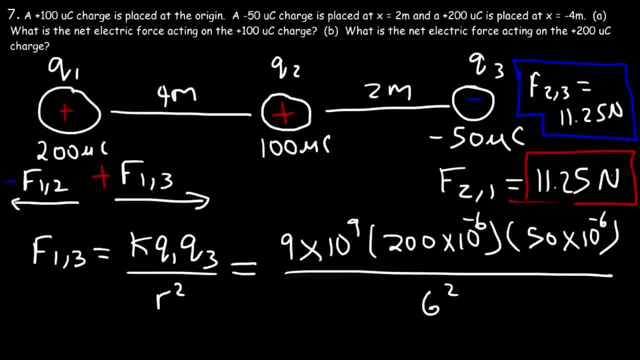 So this is going to be 6 squared on the bottom, And so the force is going to be very small. So I'm going to write it over here: It's only 2.5 newtons Because the charges are so far away. the magnitude of the force will be greatly reduced. 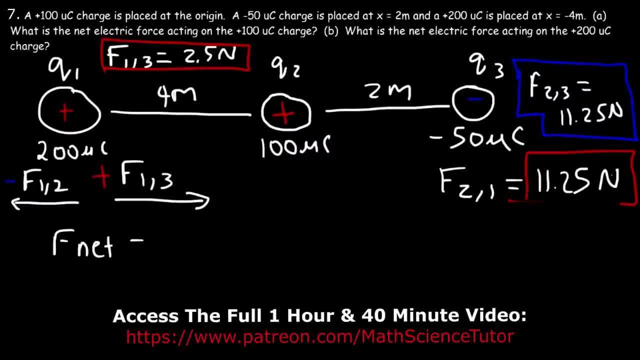 So now we can calculate the net force. It's going to be F1,2 plus F1,3.. Now this force is negative because it's in a negative x direction And it has the same magnitude as that one, So it's going to be negative 11.25.. 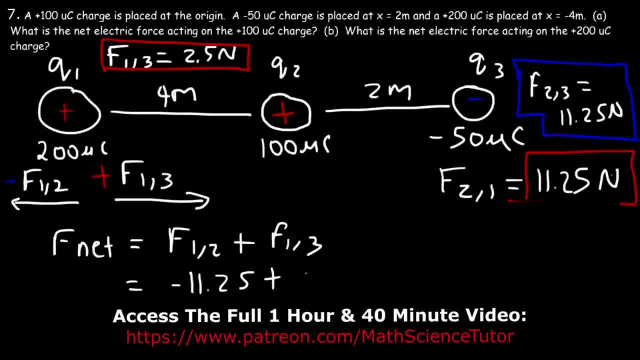 And this force is positive. It's directed in the positive x direction, So that's positive 2.5.. And so the net force is negative: 8.75 newtons along the negative x direction. So that's the net force acting on charge 1..